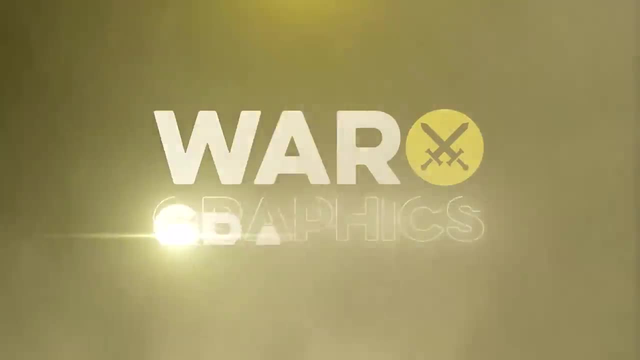 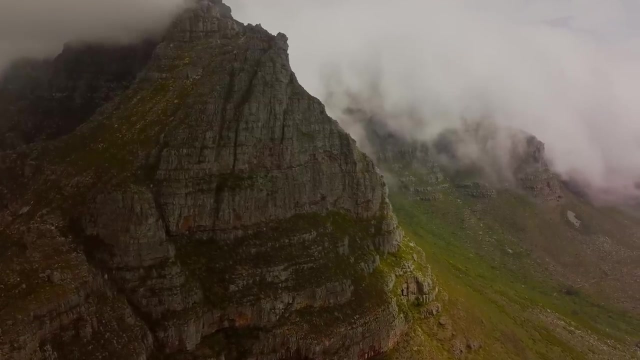 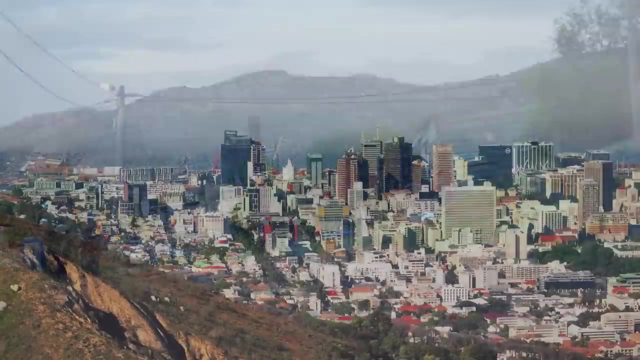 The Post-Apartheid Era. Now South Africa is a nation still trying to find its footing. After the upheaval and social reformations of the post-apartheid era, the nation has settled somewhat into a strong regional player among the most important countries of the Southern Hemisphere. 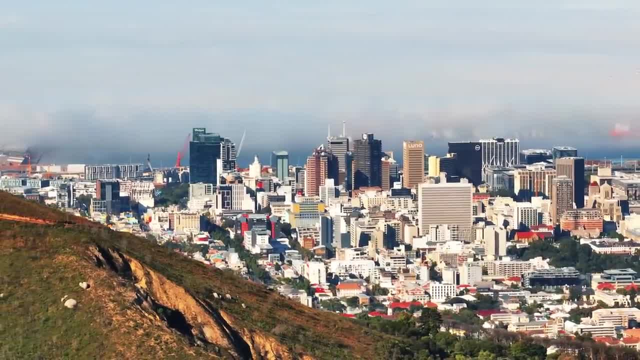 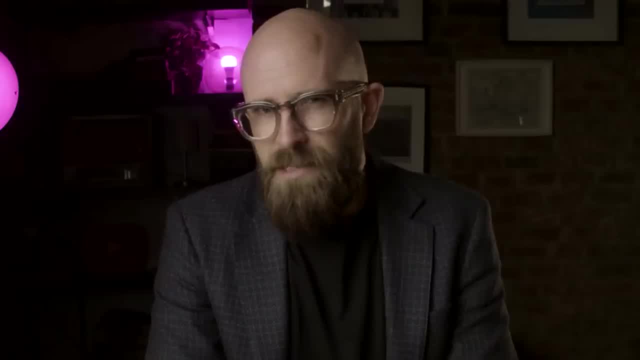 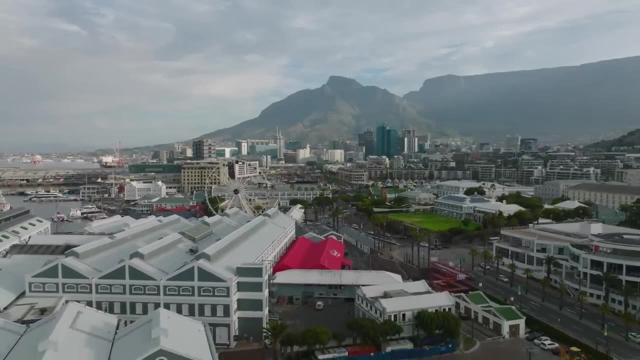 But its rapid economic growth, its rapid industrialization, its political restructuring and its complex place in the global geopolitical balance has left South Africa racing to play catch-up with its own forward advancement. Put simply, it's all well and good to enjoy a swelling economy or live through positive societal change, but when every sphere and sector are growing at once, disparities in how fast you can move forward are becoming more and more important. And as each sector grows, it's going to leave room for one inescapable influence… Corruption. 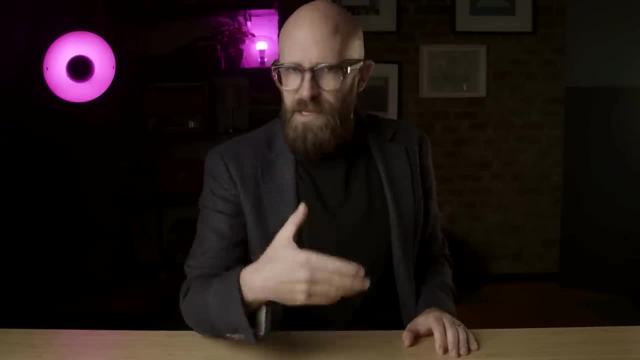 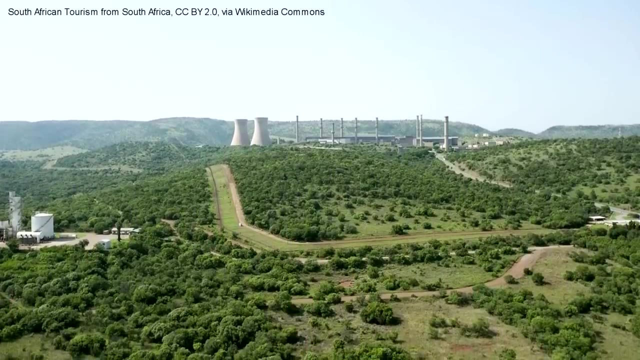 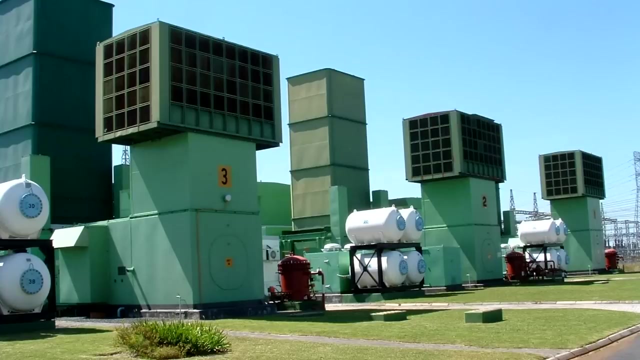 You see, in South Africa, energy has always been a complex issue. At the end of apartheid, the country found itself in a relatively advantageous position on the energy front, Bearing the weight of sanctions and forced isolation, South Africa's apartheid regime had pursued a policy of strict, nearly obsessive self-sufficiency. an initiative 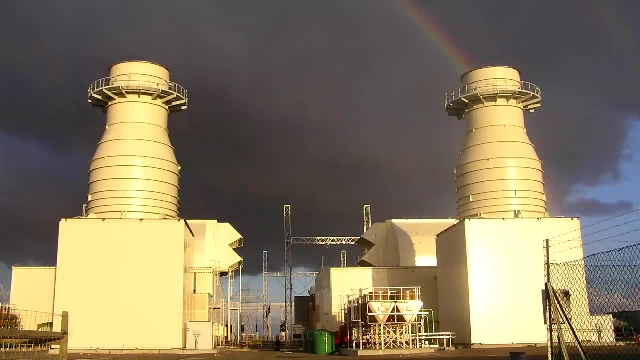 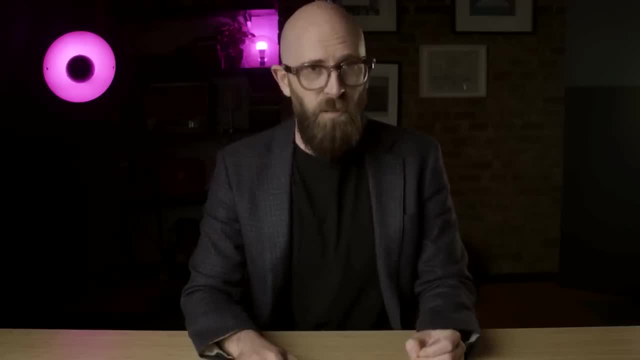 that built more than enough coal-fired power plants to keep the lights on. When apartheid ended, South Africa had more than enough electricity to power its own power plants. It had enough electricity to electrify 2.5 million households that had previously gone without, with the vast majority of those homes being lived in by black families. 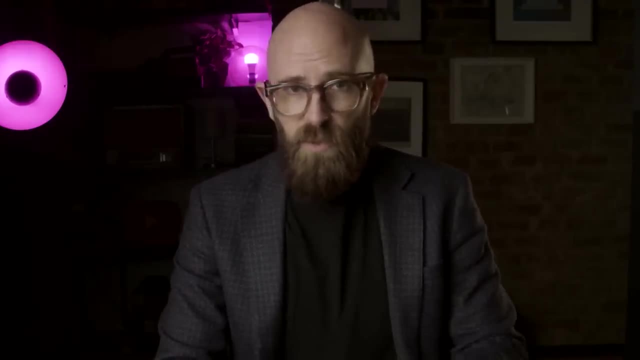 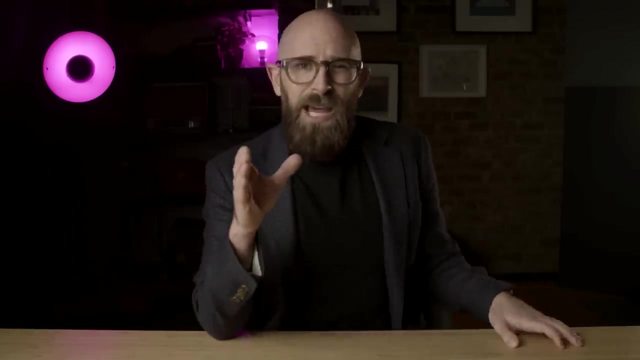 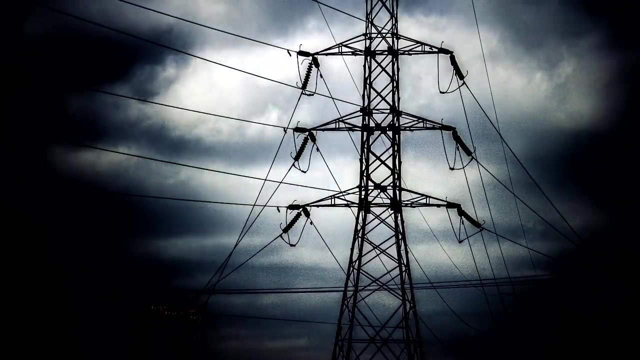 So great was the energy surplus that South Africa even began to export its electricity to nearby nations. But even early in South Africa's post-apartheid years, the country knew that it would have an energy crisis on its hands before long. In South Africa, energy utilities are managed by a company called Eskom, which is owned 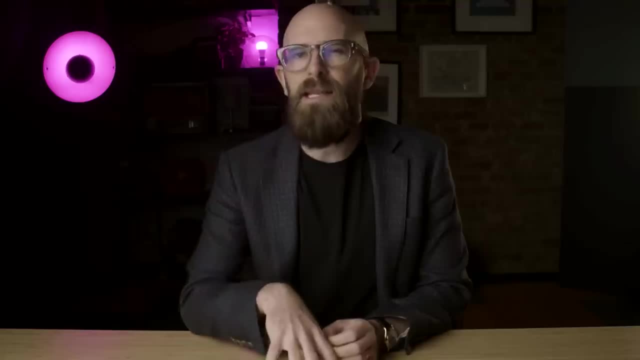 and operated by the South African government directly And as early as 1990, it was the first country in the world to have a power plant. In 1998, just a few short years after the end of the apartheid regime, Eskom had figured. 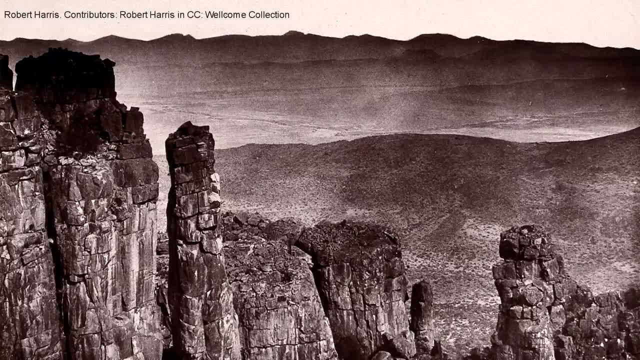 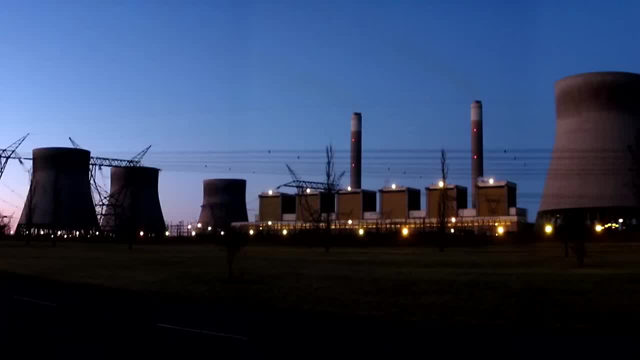 out that it was on track to run out of electrical reserves by the year 2007,. unless something changed, Eskom's older power plants were going to need to be phased out. Many of them were unreliable and the government at the time was unwilling to invest in the 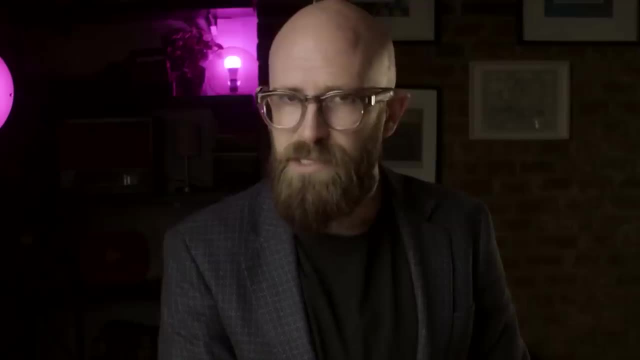 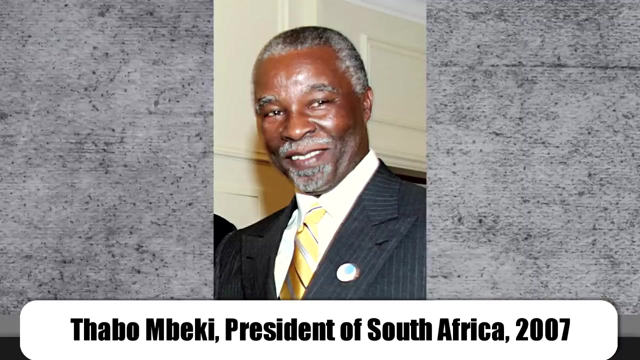 sorts of building operations that would increase Eskom's nationwide capacity. There was at that time some talk of taking Eskom into the private sector, so the government opted against taking action for years, Until it was too late. For example, There was no need for Eskom to get in front of the crisis before it happened. 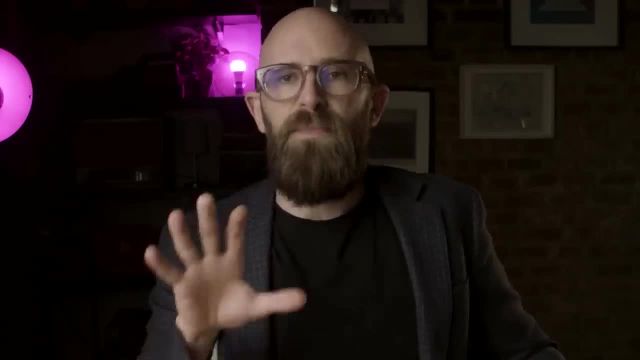 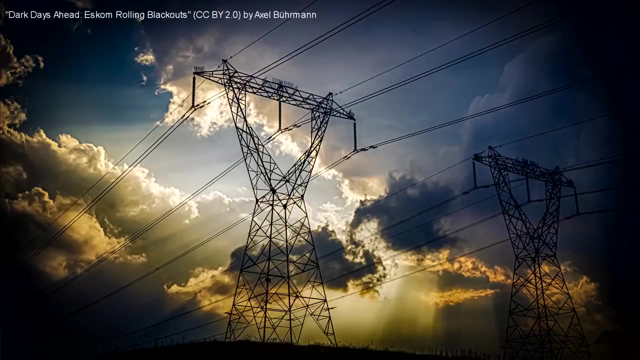 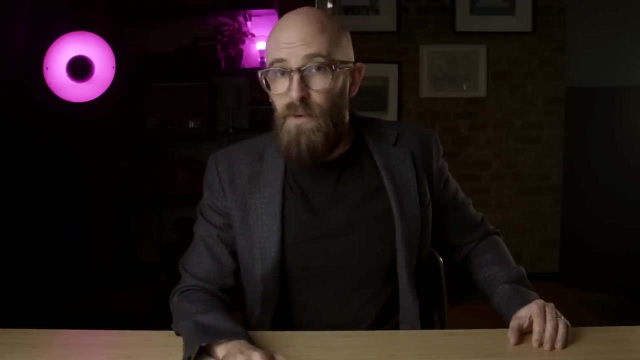 In the years since 2007,. there's one word that has become synonymous with South Africa's energy management systems: Load-shedding. This is a practice of intentionally engineering rolling blackouts to rotating parts of a city, region or country in order to lighten the load on the power system and prevent the entire thing from collapsing, With demand for electricity in South Africa still rising as more homes come onto the grids but barely any meaningful supply increase. In fact, there's no need for a power plant in South Africa. The power plant has been a major problem since 1996, and rolling blackouts have become 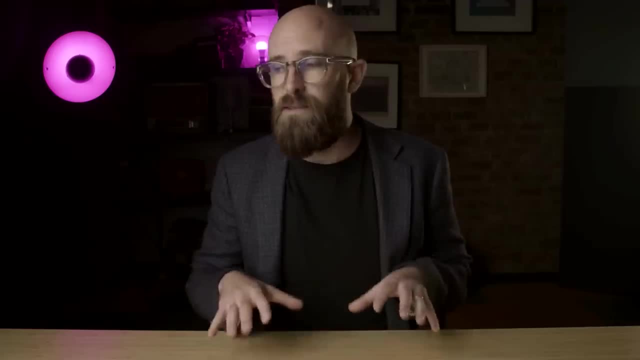 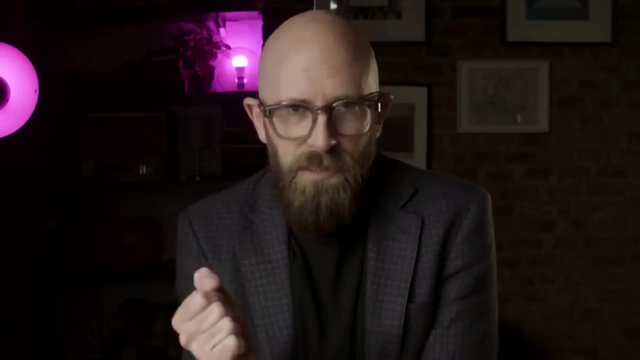 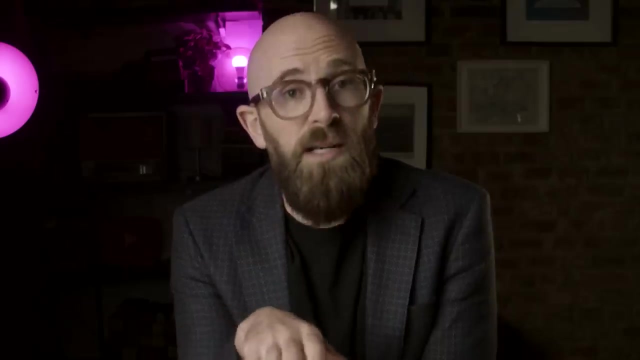 an absolutely necessary step to keep South Africa's lights on at all. Add to that, the fact that most of South Africa's power plants are now aging badly and need constant maintenance means that if a plant breaks down or needs to come offline for some reason, the need for load-shedding only gets worse. 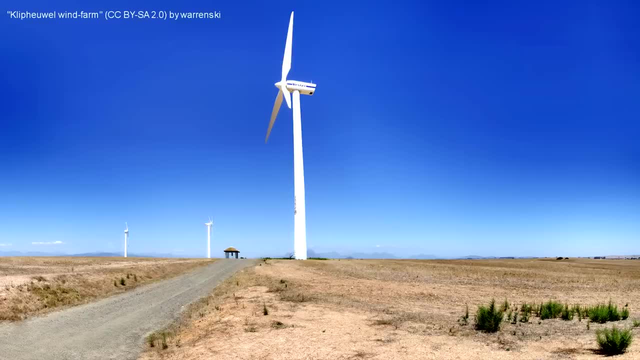 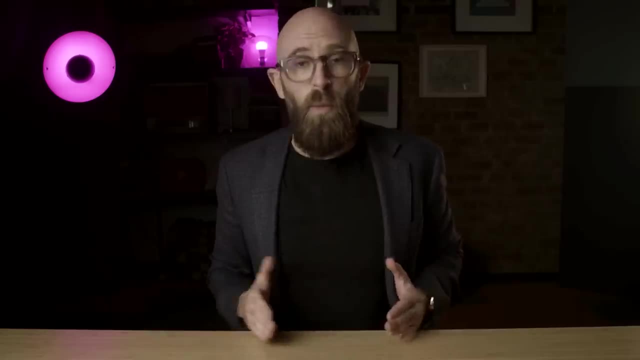 For well over a decade now, this very public issue has made Eskom and South Africa's energy infrastructure into a lightning rod, Not just for public criticism But for the use of power, For the use of furthering the goals of a wide range of players within South Africa. 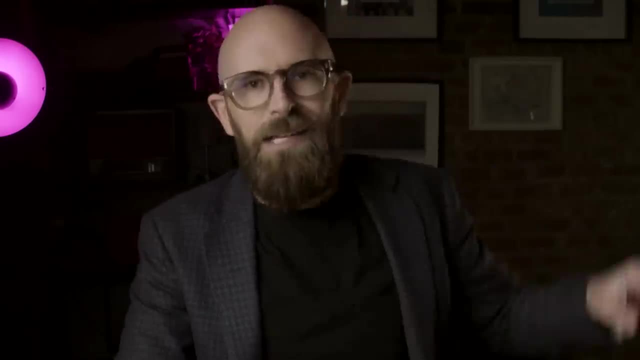 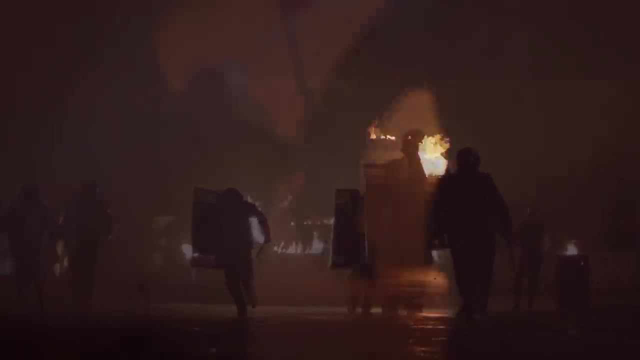 If a politician wants to score some easy points, they can dunk on Eskom. If labor unions at Eskom's power plants want to strike, they can leverage their ability to disrupt the nation's power supply. And if violent actors, saboteurs or terrorists want to hit the government where it really, 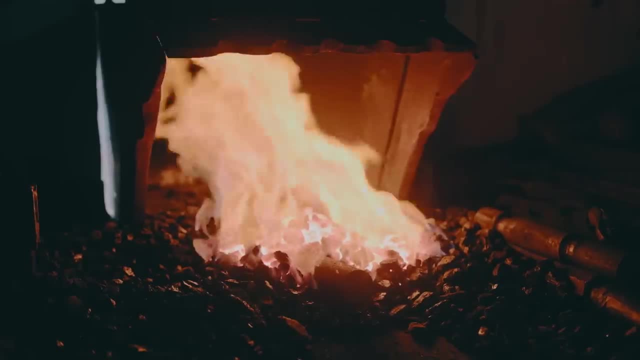 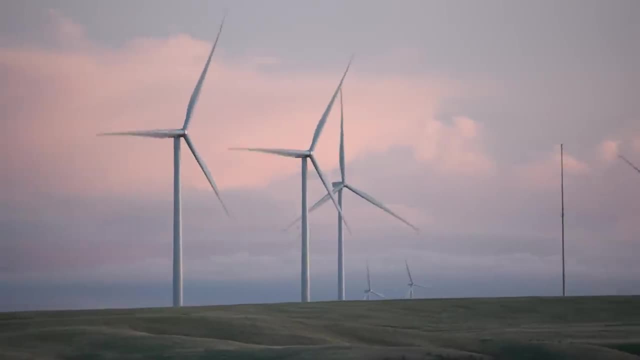 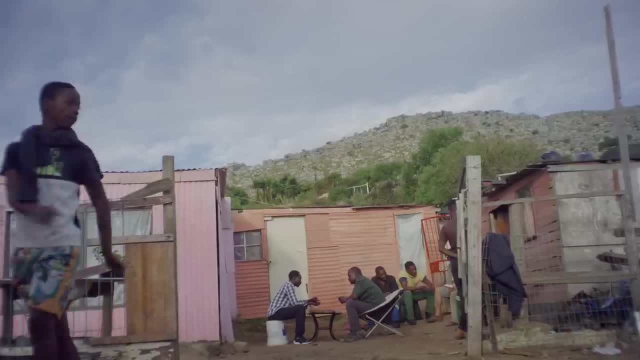 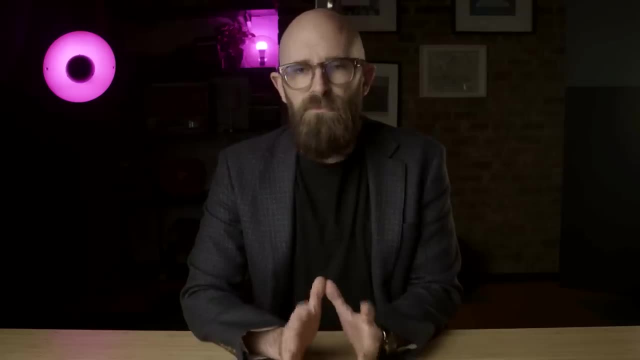 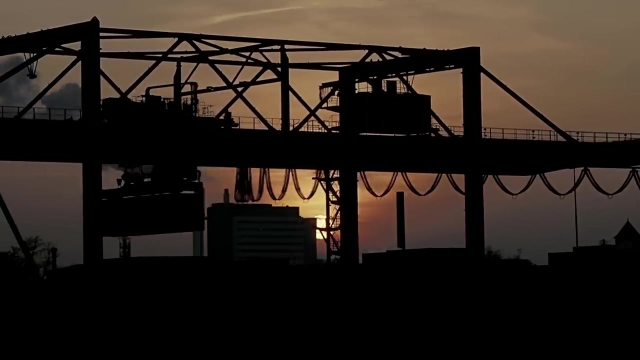 Now today, in the early 2020s, the problem is only getting worse. Some South African households experience nearly half a day without electricity on average, And the country's once booming industrial sector has been forced to cut costs, cut corners and deal with the expectation that blackouts are all but unavoidable. 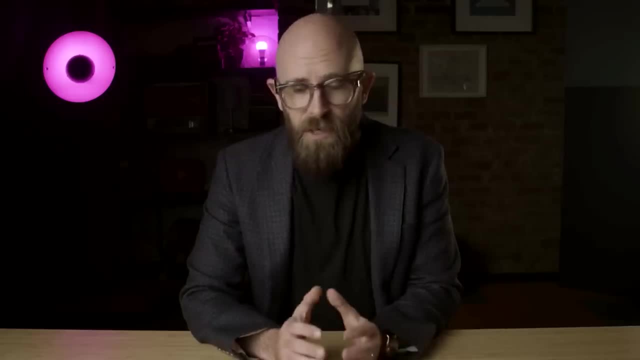 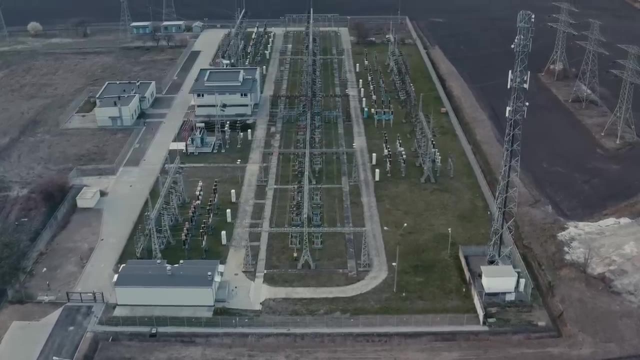 South Africa has continued had to ramp up the severity and the extent of its countermeasures against the drain on electricity to the point that well over a third of the country's electrical grid may go without power for part of a given day, after a series of breakdowns in over half a dozen power. 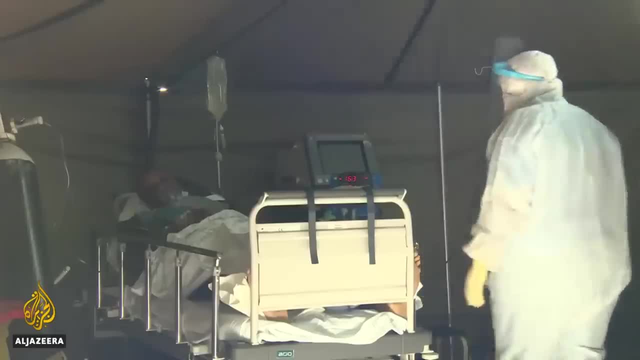 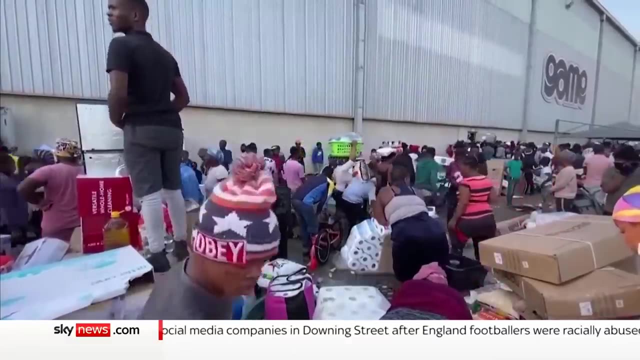 stations forced load shedding to be reinstituted. during the covert 19 pandemic, things have simply never gone back to normal, and strikes, environmental catastrophes, fires and more and more frequent breakdowns have escalated the situation even further. in 2022, south africans dealt with load. 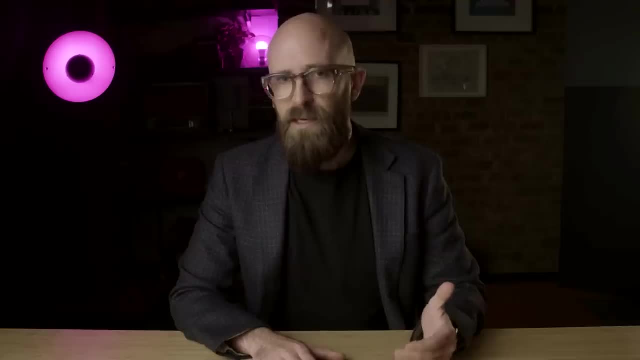 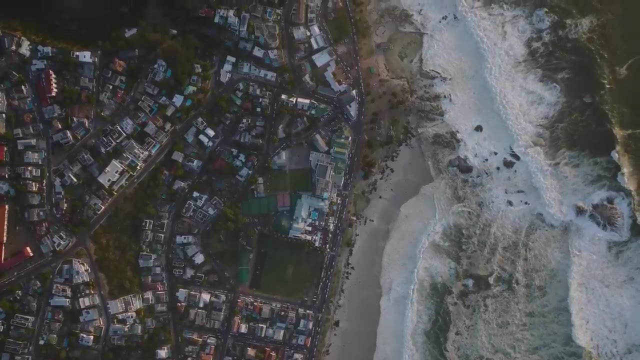 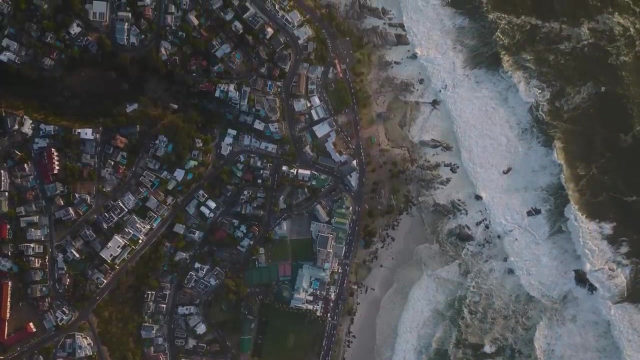 shedding measures for over 200 days out of the year and 2023 so far has made 2022 look a bit like child's play now, as bad as south africa's situation probably sounds already. we've got to make it clear that the nation's energy crisis does not exist in a vacuum. instead, south africa's 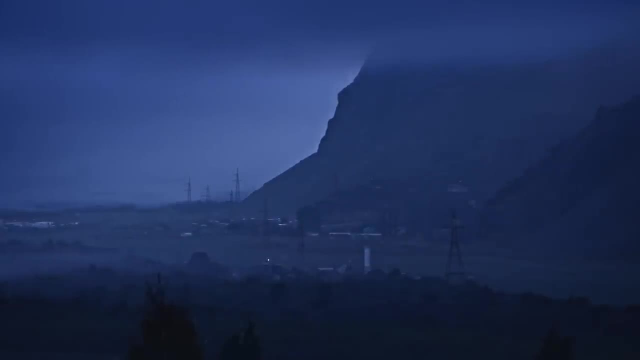 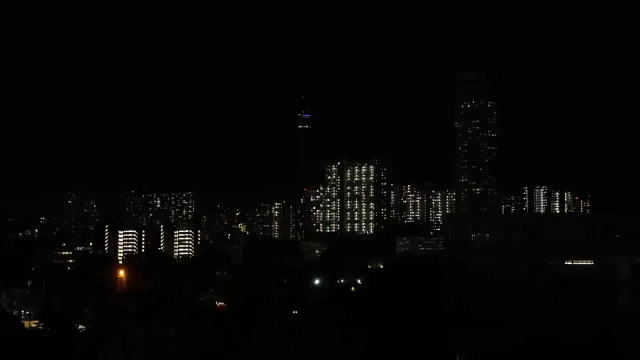 rolling blackouts are either a symptom or a cause of a wide range of other issues facing the country, issues that seem to get worse and worse as the blackouts continue. now, first, there's a problem that both bears the blame for the crisis in the first place and has meaningfully 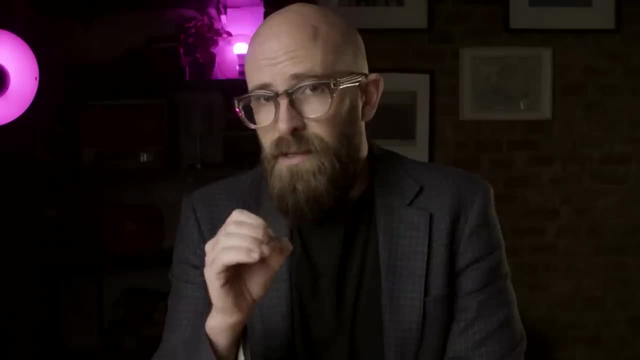 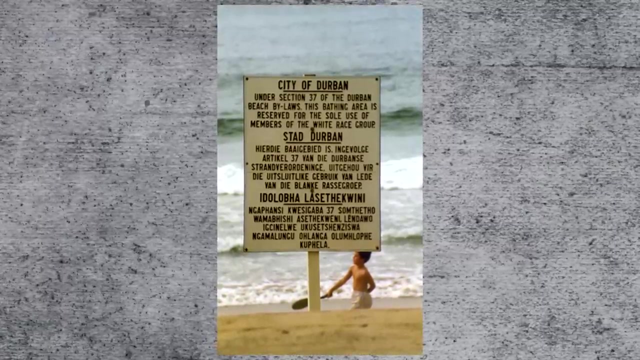 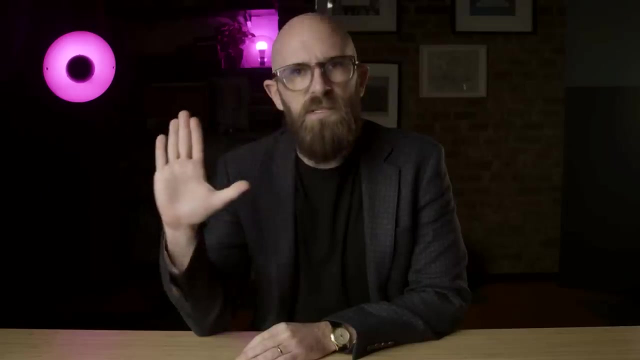 accelerated the race at which things have gotten worse, and that is corruption, something that south africa has had rampant problems with from its apartheid days to the immediate aftermath. till today, south africa has robust laws in place that are supposed to deal with corruption in all spheres but enforcement. 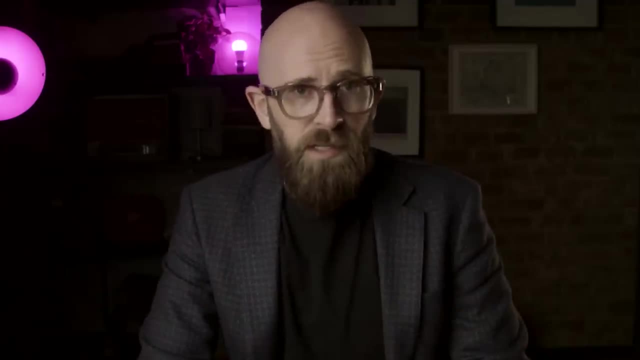 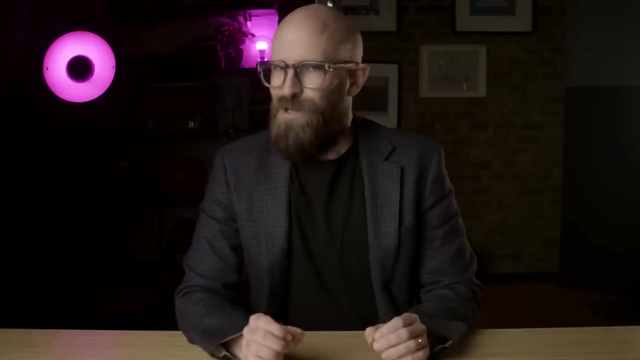 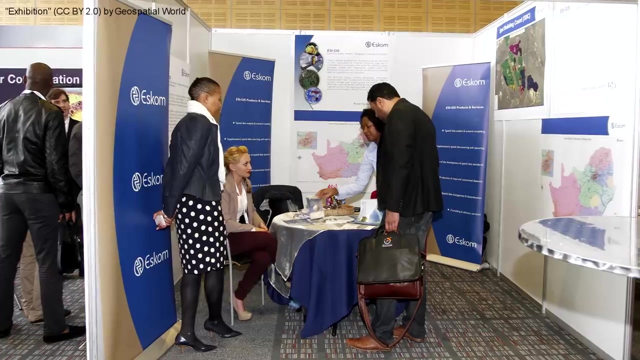 those laws has been lax for decades, a problem that got even worse under the tenure of president jacob zuma, who led south africa from 2009 to 2018.. perhaps not so coincidentally, those were years that the energy crisis could have been dealt with, but just wasn't. the escom utility has its own fair. 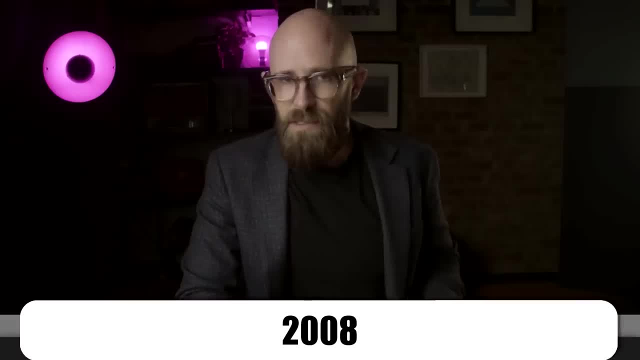 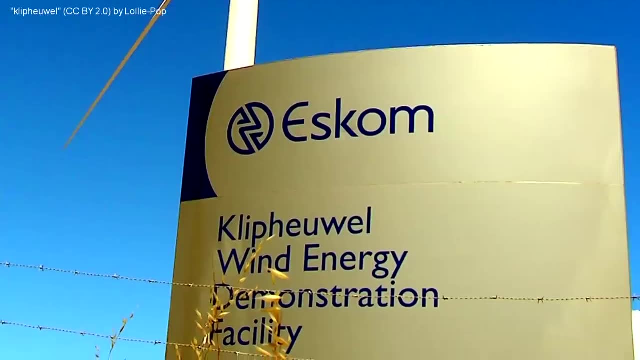 share of corruption, with a long list of scandals beginning in 2008 and accelerating significantly in the years of the covert 19 pandemic and afterward. in some cases, this is as simple as escom employees taking bribes to sabotage their own facilities or open the gate so that diesel oil thieves can. 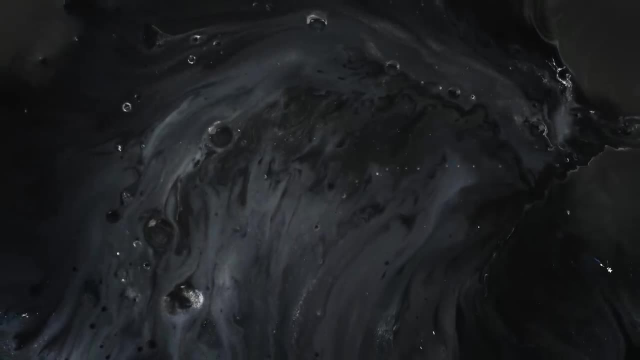 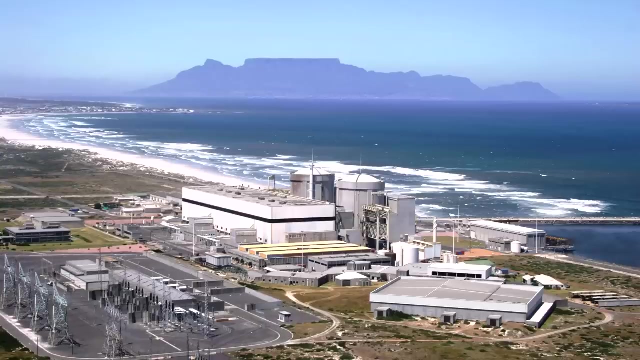 sneak in and make a heist. in other cases, officials have routinely lied or obscured the low quality of coal used in plants, while outside actors, particularly repair companies, have arranged parts of power plants to be stolen so that they can be called to fix the problem. escom's own former. 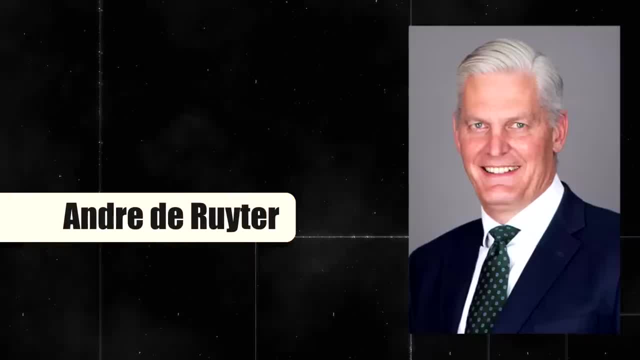 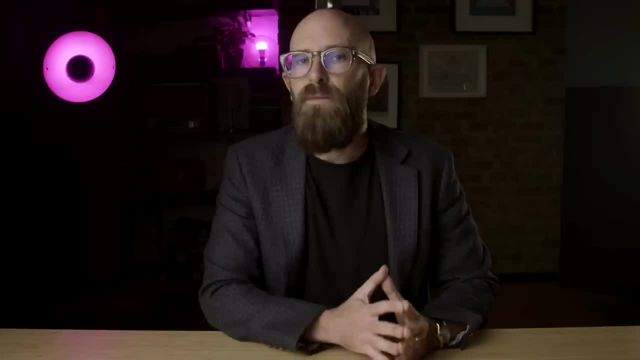 ceo, a man named andre de ruta has alleged that the company is deeply infiltrated by chemical syndicates, with high-level officials directly in the country and the government is not able to involve, and that corruption siphons away the equivalent of over 50 million us dollars from. 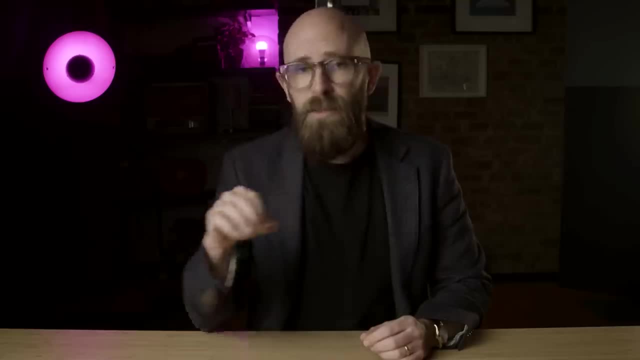 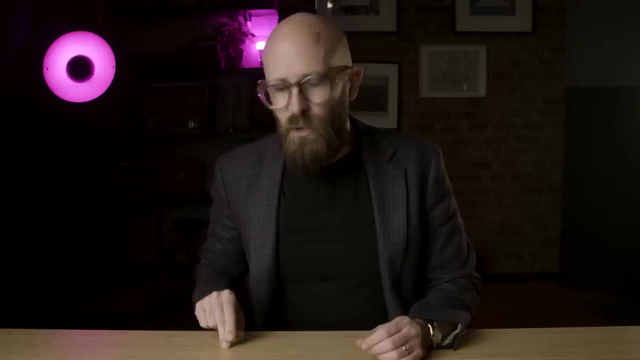 escom annually, and the two power plants that have been brought online since the start of the energy crisis, called madupi and kusile, are believed to have been rife with their own corruption during the construction process. further acts of sabotage take place with a shocking frequency, with everything. 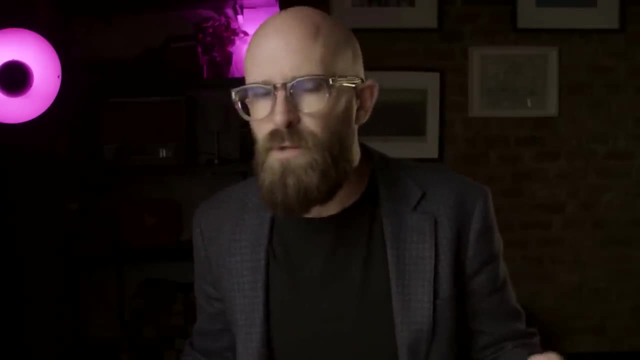 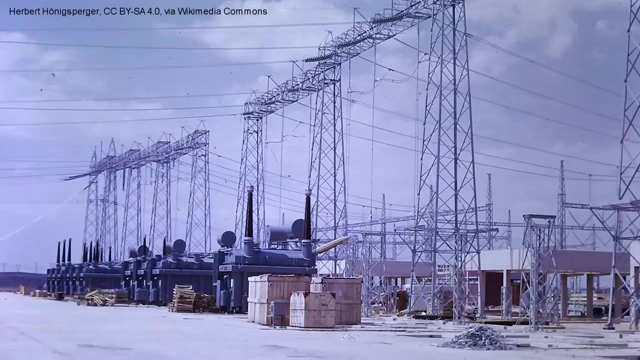 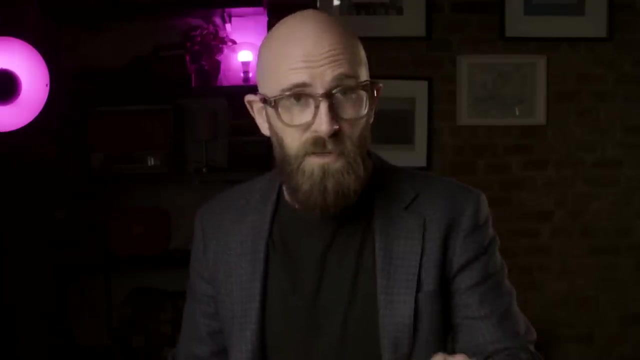 from steel supports to cables, to fuel supplies, to coal, moving infrastructure taken out of commission for a quick buck. and of course, every time saboteurs bring a power station offline, the load shedding problem only gets worse. and then there's the effect of frequent but unpredictable power cuts. 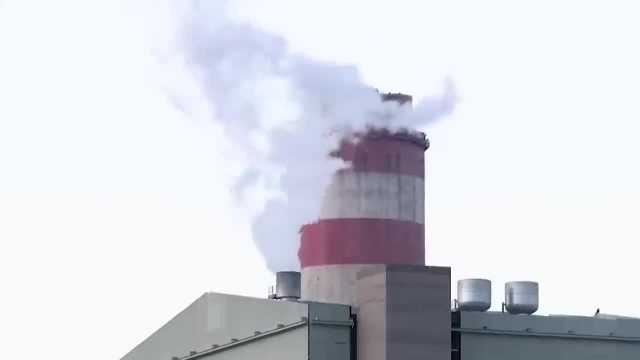 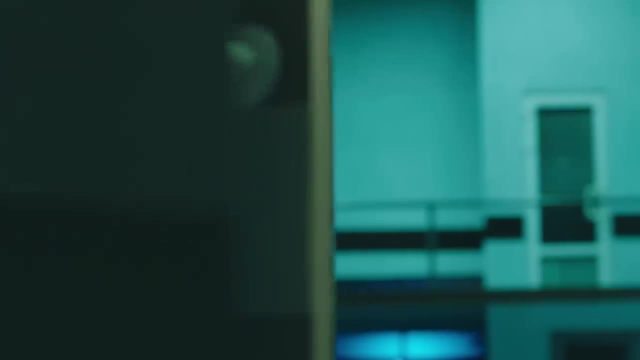 on those who are most vulnerable and, in particular, those desperately in need of treatment at south africa's hospitals, even without the power supply to worry about. south africa's public health care system is badly underfunded, it's badly understaffed and it employs doctors and nurses who are badly. 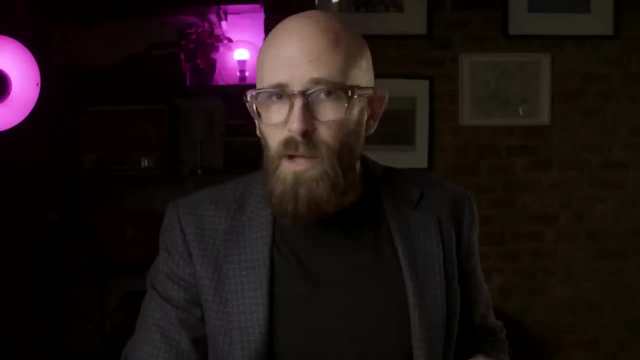 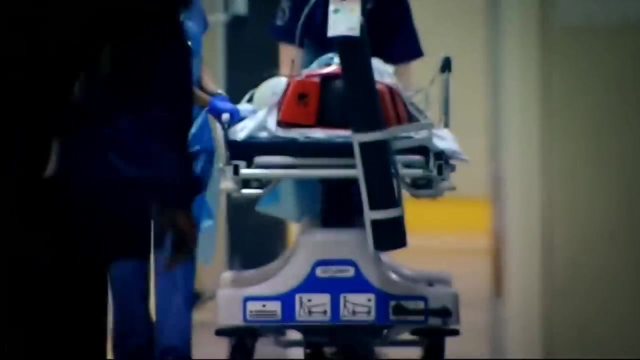 overworked, and they are dealing with all of this while being forced to deal with shortages of critical equipment and medicine. private hospitals and university hospitals are much, much better but unaffordable for most of the population. add in the energy crisis and now these hospitals are sometimes. forced to endure over a hundred hours per month without power, forced either to rely on expensive emergency generators or just take the risk that people will die who are attached to essential equipment like ventilators when the electricity goes out. patients in operating theatres are at exceptionally high risk, as are infants in neonatal intensive care units and 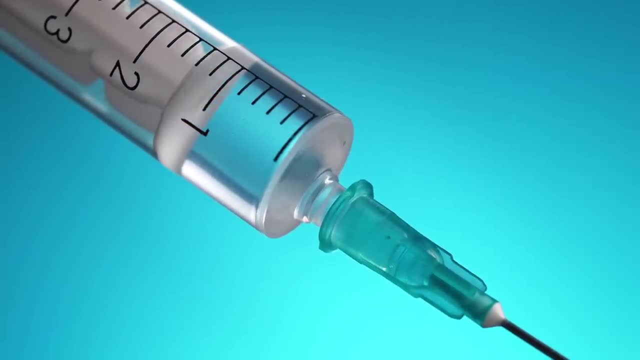 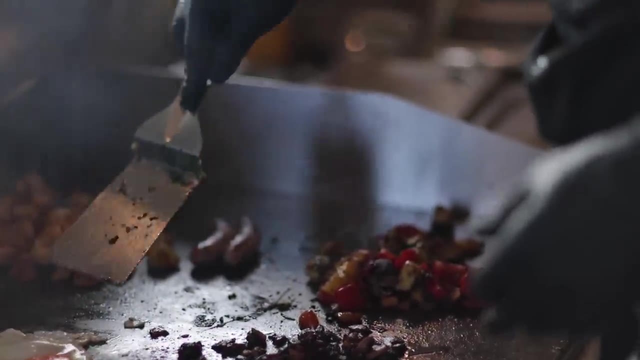 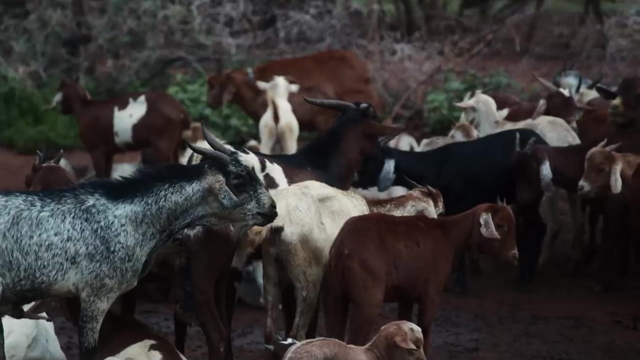 many vaccines and medicines that must be refrigerated are useless by the time the power returns. when it comes to south africa's food sector, the situation's no better. power cuts wreak havoc across the nation's food infrastructure, from meat to dairy products that spoil on mass with a lack of refrigeration, to the large-scale die-offs of livestock raised in enclosed factories. 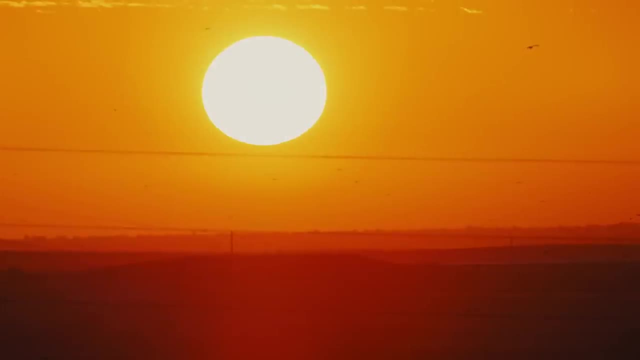 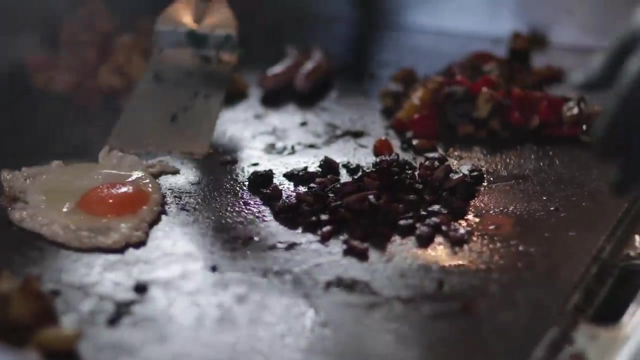 due to heat and a lack of ventilation. with availability of food supplies and food supplies of food so tightly restricted, prices skyrocket, taking much of the nation's regular diet out of the reach of its ordinary citizens, and the same goes for produce: it wilts and it rots before it. 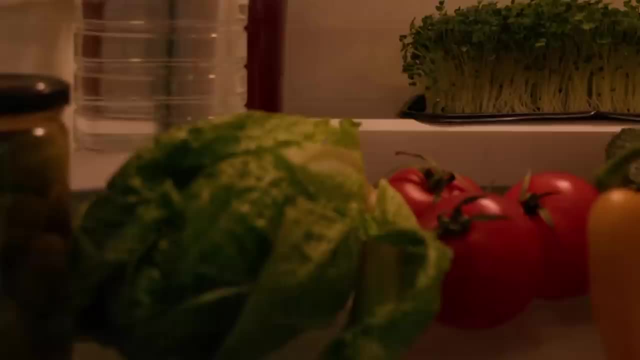 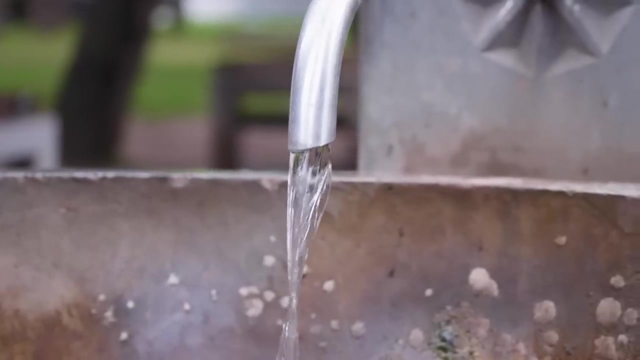 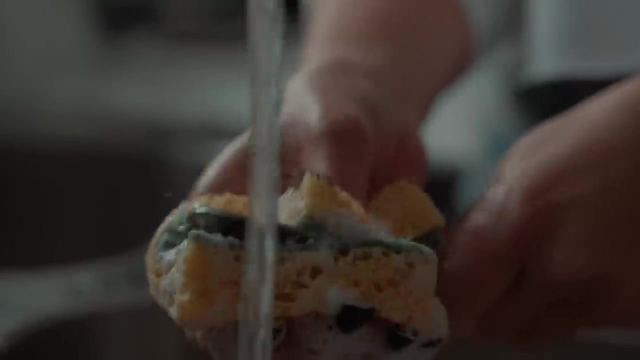 can ever grace a dinner plate and staple ingredients that should otherwise be able to last for months in people's refrigerators are just wasted in the last few months, even south africa's taps have started to run dry, with not enough electricity throughout the day for functions even so essential as pumping water into homes and businesses. 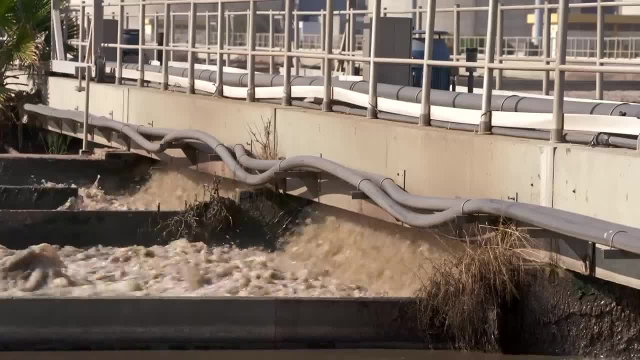 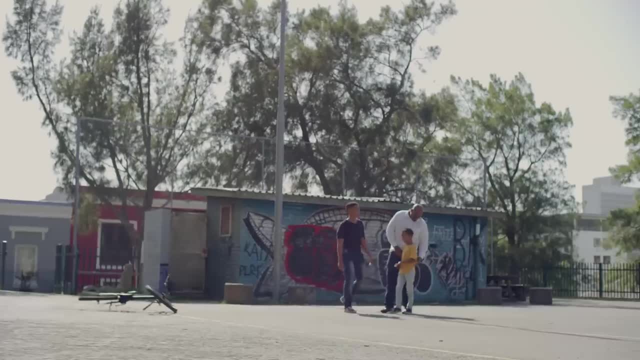 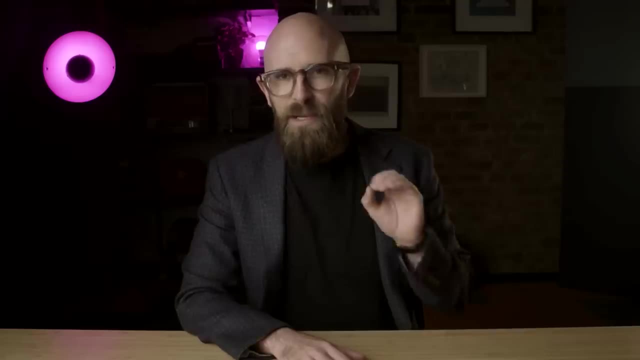 after that, the power cuts his impact on sewage treatment plants, ability to clean wastewater, and soon there may be no guarantees that even the water that does reach somebody's home is safe to drink. and then there's the south african economy, where unemployment has reached staggering highs of 33 percent nationwide. that figure is so high for a wide range of reasons, but among them 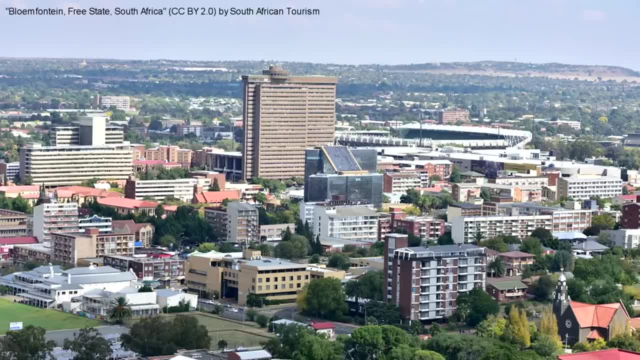 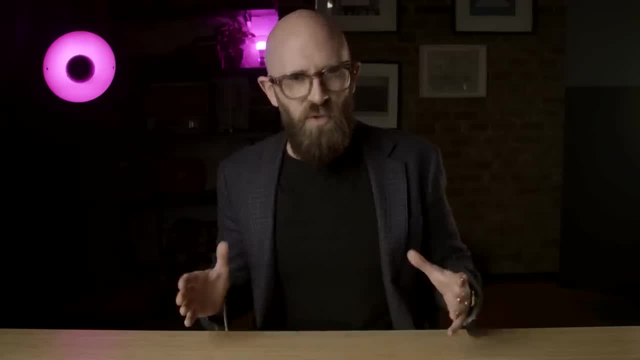 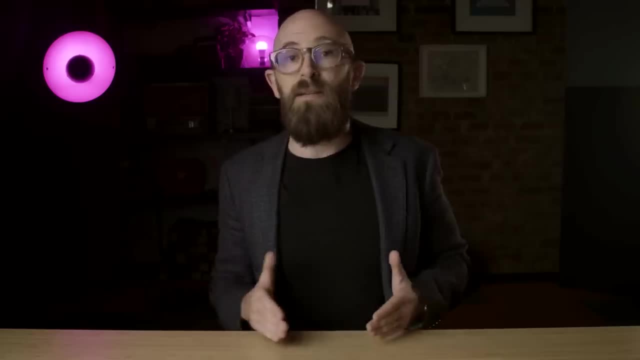 is the simple fact that many businesses in south africa or any other nation will need a stable energy supply in order to remain at work. small businesses who depend on power to operate are left hung out to dry whenever load shedding impacts their districts, often making large parts of the business day functionally useless. while ensuring that any 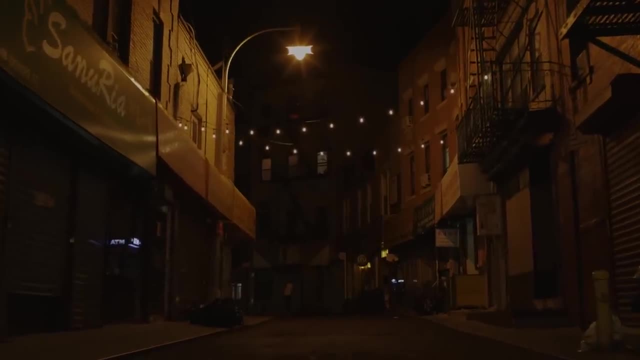 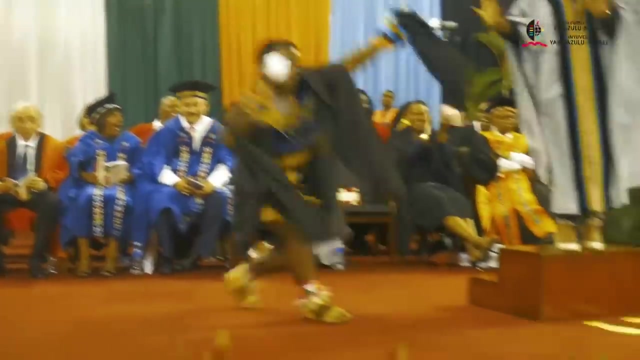 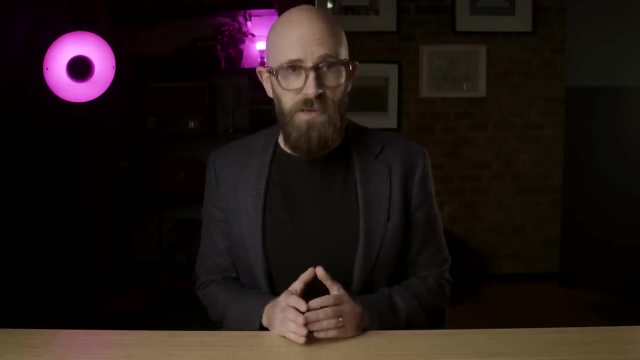 moments in which the power is on is a mad dash toward whatever productivity they can manage. many companies have stopped hiring in anticipation of worse pain to come, meaning that young south africans are more and more frequently entering a workforce that just has no place for them. on a larger scale, south africa's central bank estimated that the nation's load shedding 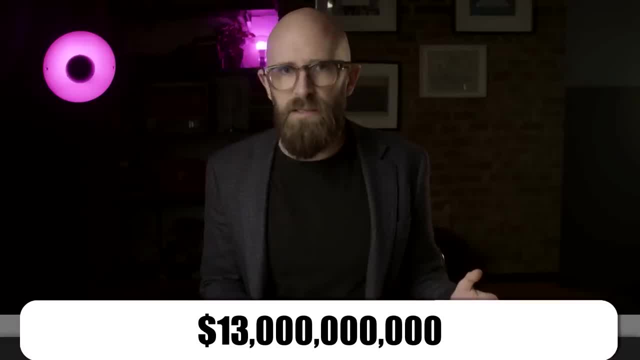 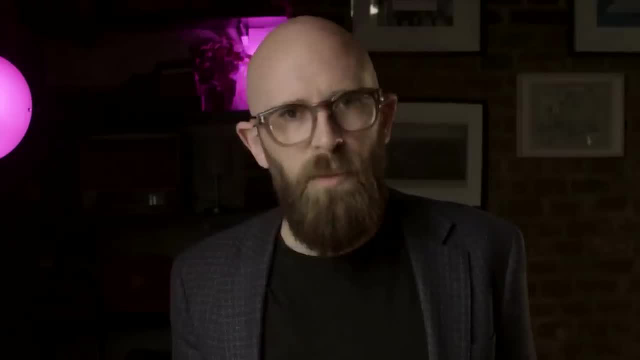 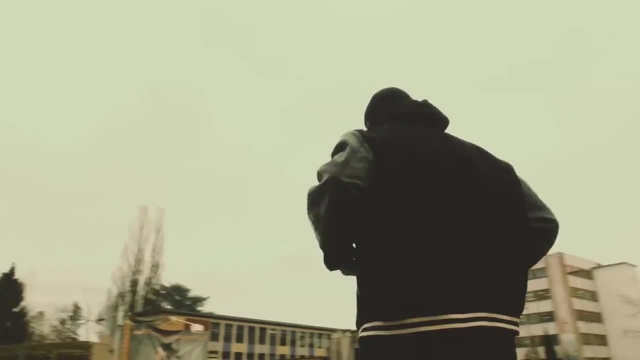 policy would inflict costs of 13 billion dollars on the country's economy, and the country's gdp growth continues to fall towards zero. and finally, we just have to talk about crime. in regards to break-ins, burglaries, larceny, looting, power outages present a prime opportunity for criminals to do. 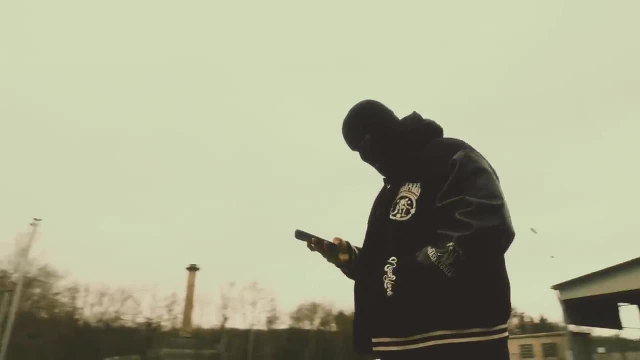 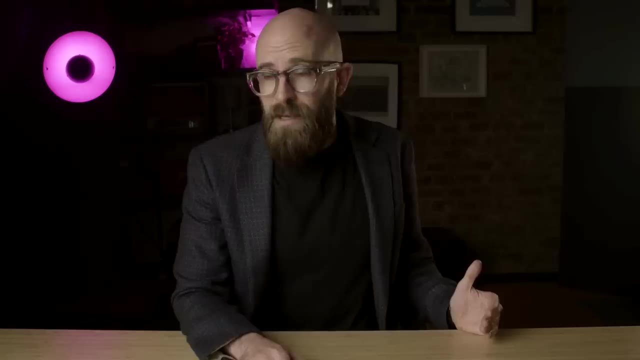 their work unopposed with electric fences, alarm systems and street and indoor lights- all inoperable now. the country's crime rates were already high prior to the recent low jetting increases, and they've now gone through the roof, while the plight of some of the most vulnerable communities in the 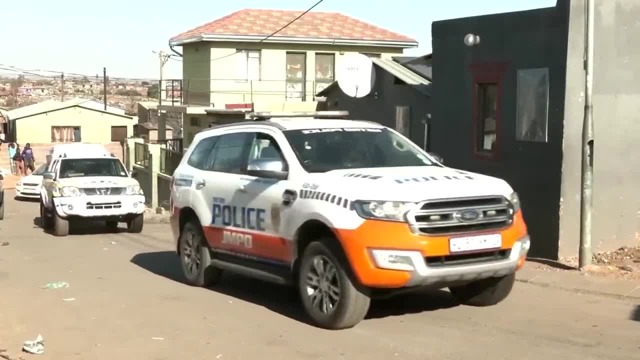 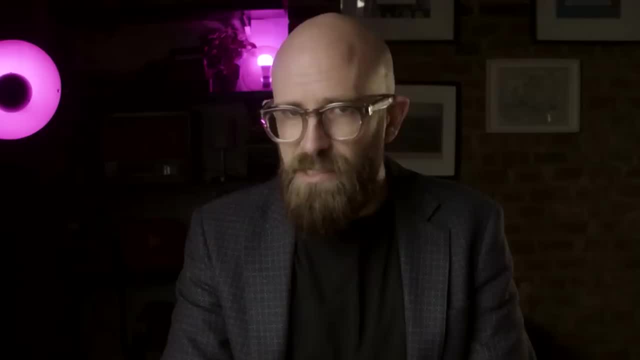 country is at a low level of crisis and the police are less able to respond to homes and businesses seeking help. and that's not just because of communication interruptions either. with traffic lights rendered inoperable, police have to fight their way through badly congested streets in order to get anywhere. political violence is also on the rise, as protesters 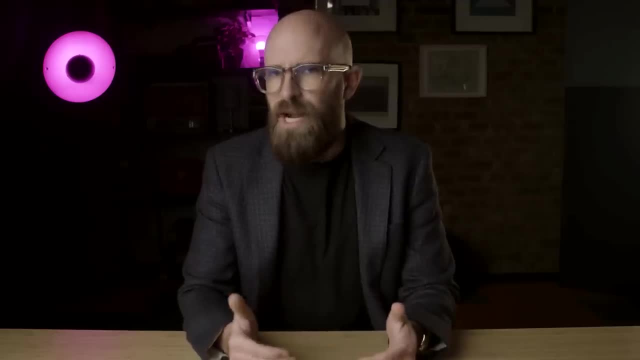 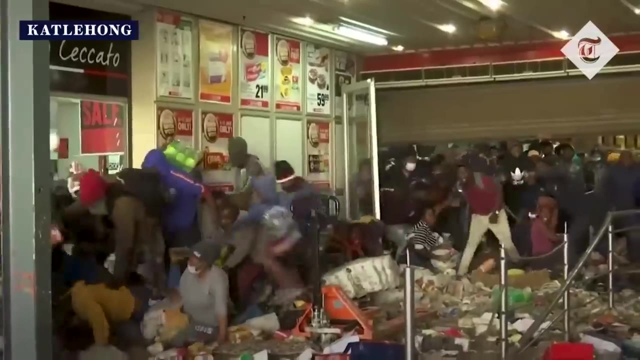 and discontented civilians begin to feel more emboldened to take drastic measures in order to make their voices heard. some of south africa's biggest cities have witnessed protests turn to violence and then to riots. so when trying to figure out just how much money we're spending, 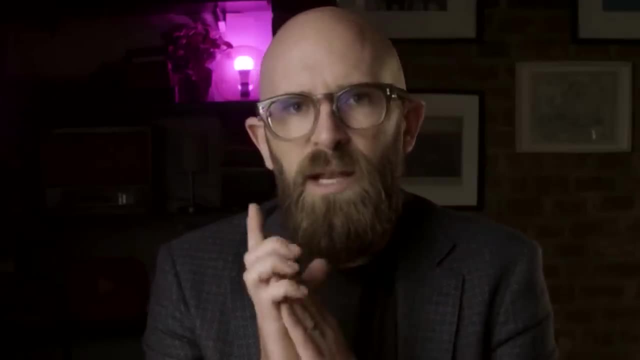 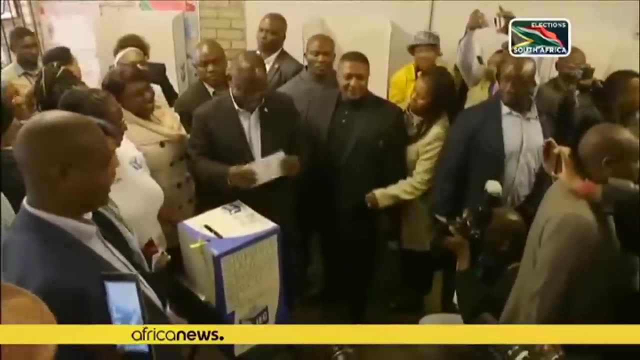 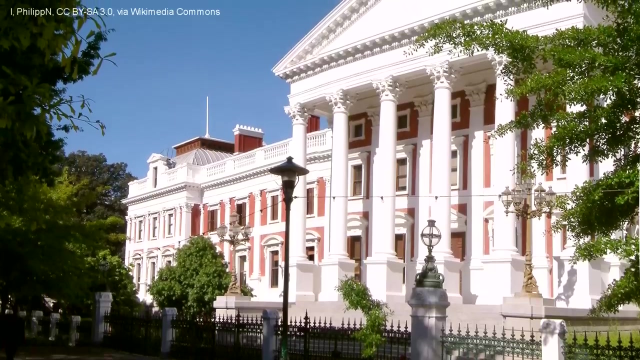 and what all of this means for south africa. there is one clear and uncomfortable reality. to start with, south africa is rolling into election season. these elections, held in 2024, will contest all 400 seats of the south african national assembly, where the african national congress anc. led by south 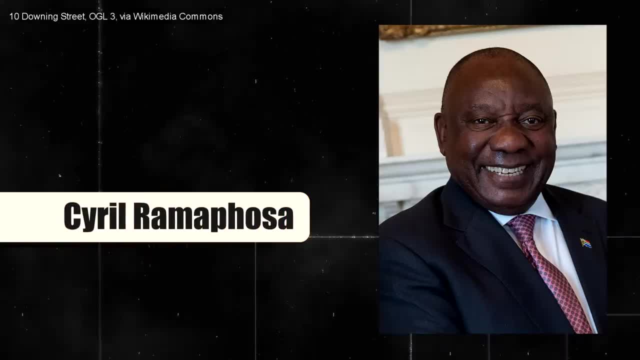 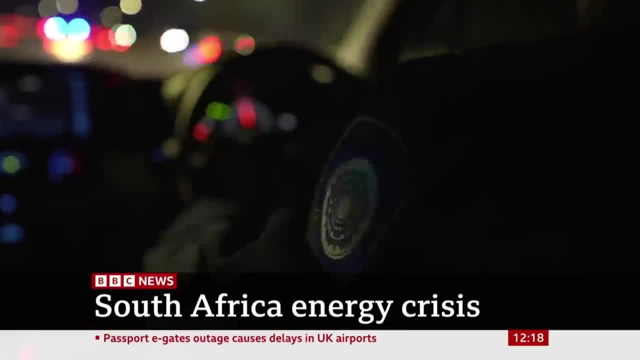 african president, cyril ramaphosa, has held a controlling influence for the vast majority of the country's post-apartheid history, but in 2021's municipal government, the african national congress and the municipal elections, the anc suffered a warning shot across the bow with the party. 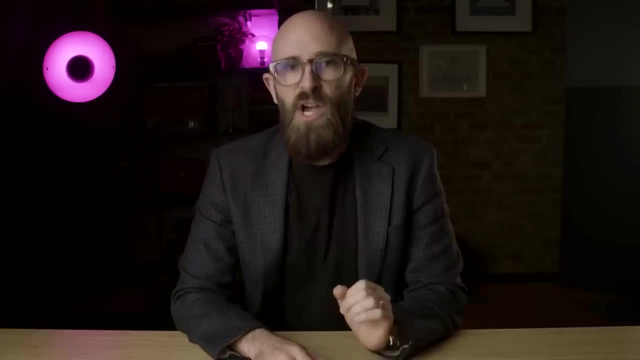 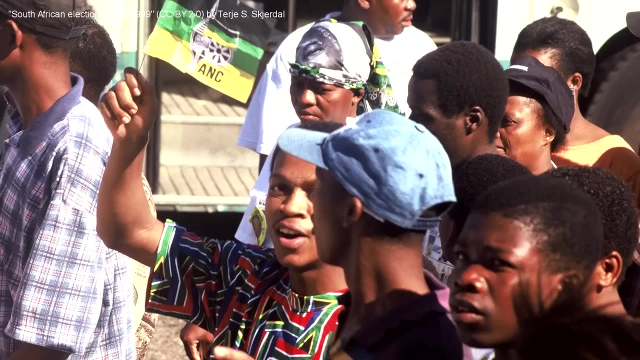 receiving fewer votes than ever and suffering a significant ongoing hit to approval ratings. now look, it would be premature to declare that the anc is on its last legs. the party still has a good chance to receive a plurality or even a majority of votes in the 2024 elections, but with the nation's many opposition parties conspiring more closely than ever to form a coalition. there's also a fair chance that the anc, even with help from other parties, will have tried to win the election in the last few weeks of this year's presidential election, and that's. 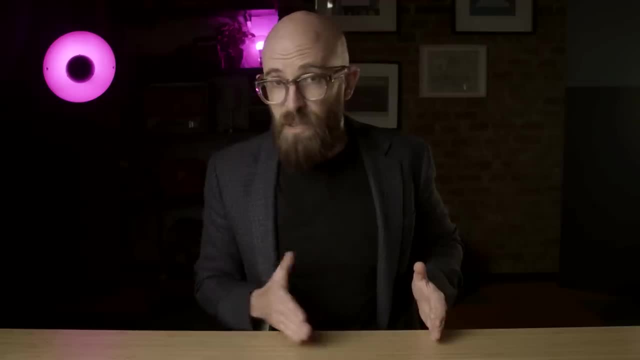 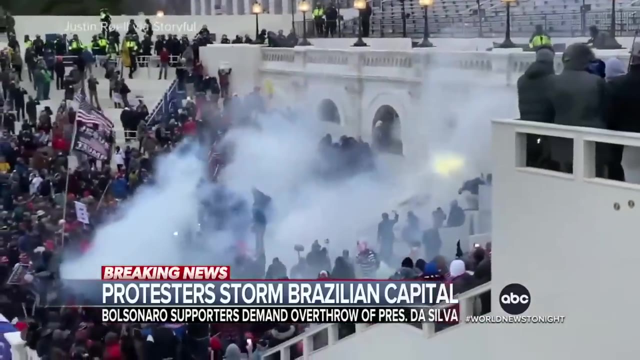 the only way to get the majority it needs to govern. perhaps the worst possible outcome is one that would take a page from the aftermath of the us 2020 presidential election or the 2023 riots that took place in brazil after president jair bolsonaro was voted out of office under such 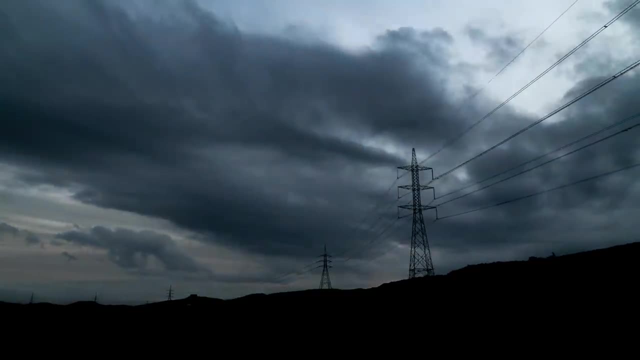 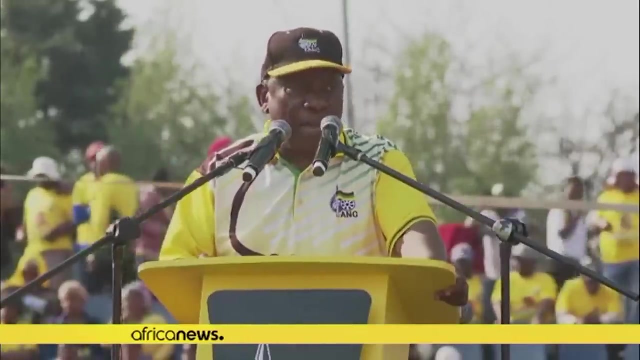 pressure from the blackouts and from the many, many issues that follow on from them. it's not inconceivable that a close or conspiracy-fueled election cycle could be the spark to set off the entire power of the african national congress. the anc and the african national congress are 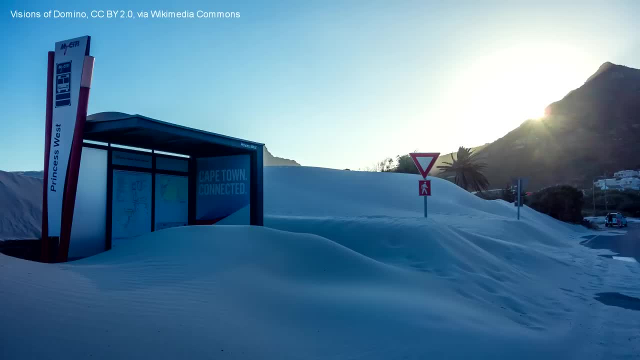 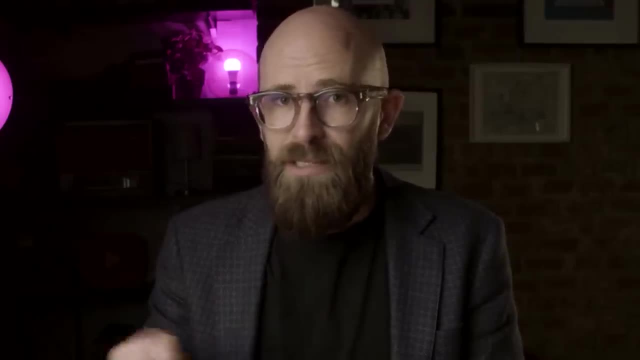 going to have to wait and see what happens in the next couple of weeks. the nation was able to weather its difficult winter season without a complete collapse this year. reminder to our northern hemisphere viewers that may, june, july and august are the coldest months of the year, not the warmest there. but just because south africa survived this year doesn't. 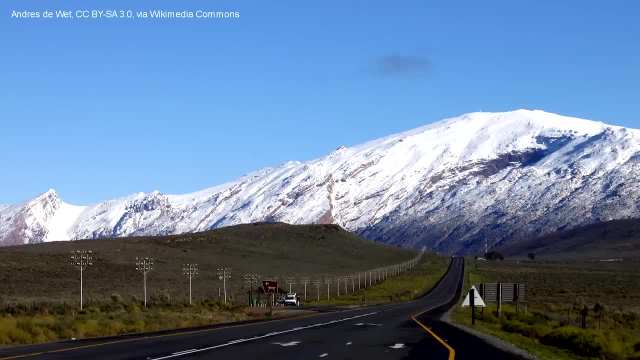 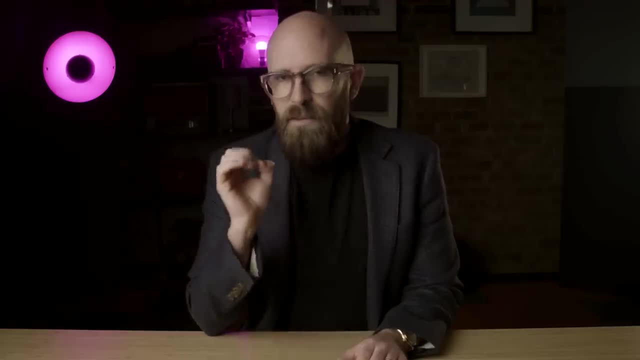 mean that it's going to have an easy time next time around and, with the date for the 2024 elections not yet set as of the making of this video, there's a real threat that continued deterioration in the country will produce an even greater threat to the african national congress. 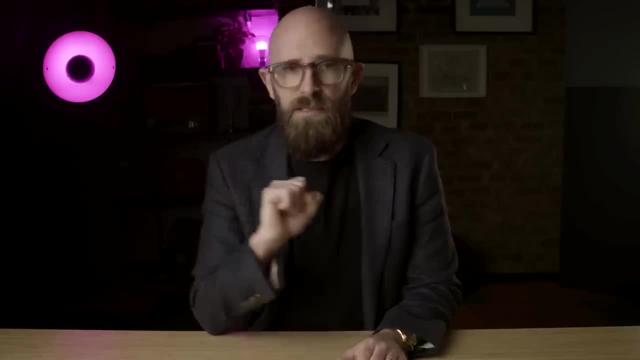 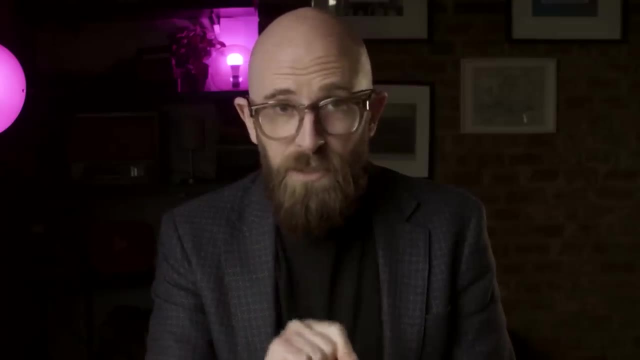 even worse, winter, right before or even during the election season. and then there's the international side of the issue, where south africa's predicament has wide-reaching ramifications, both for the country itself and the entirety of sub-saharan africa. of course, the nations that rely on south 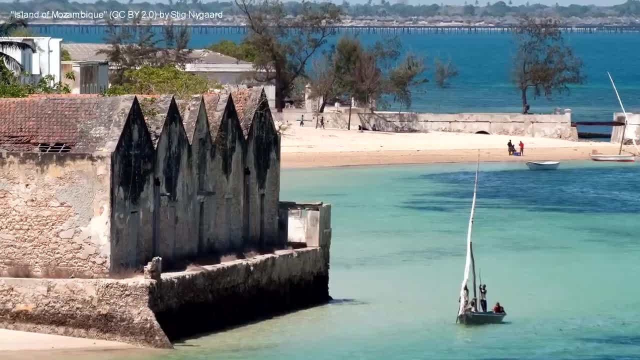 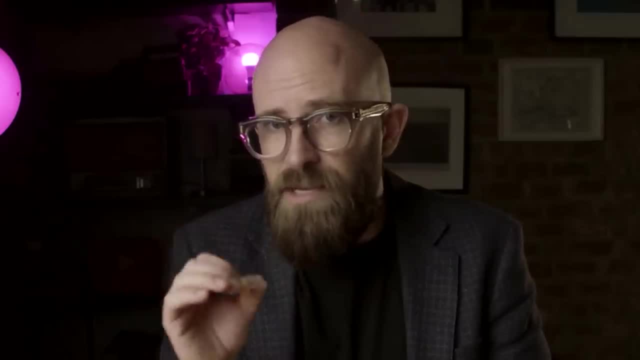 africa for their own electricity, including zimbabwe, mozambique, espotani and others suffer chronic power cuts and shortages as well, and we don't want to undersell the serious impact of those measures on those nations, even if the political problems that come from them are somewhat. 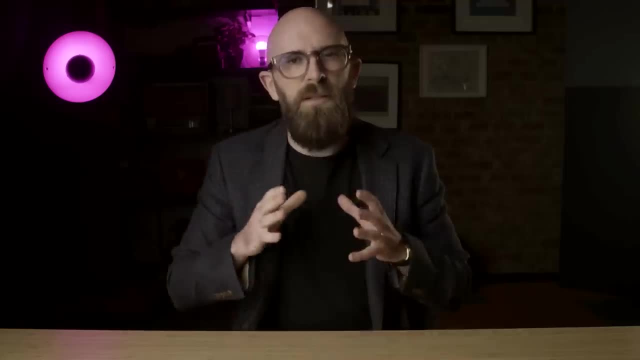 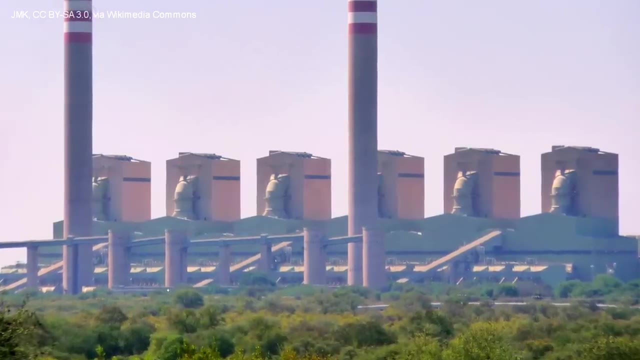 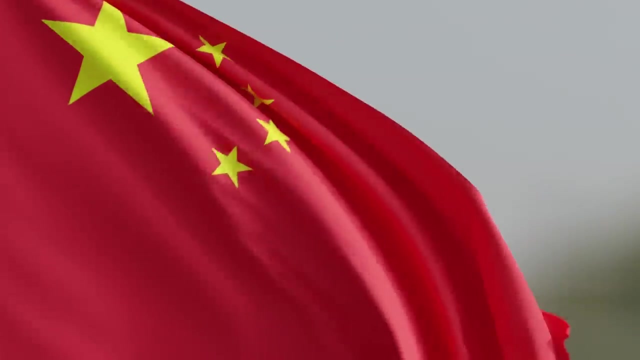 removed from south african politics, but potentially the much larger issue in a geopolitical sense is how south africa's energy crisis can be used as leverage by power players in the global community, and it's here that we mention china. china is the nation that appears most interested in being south. 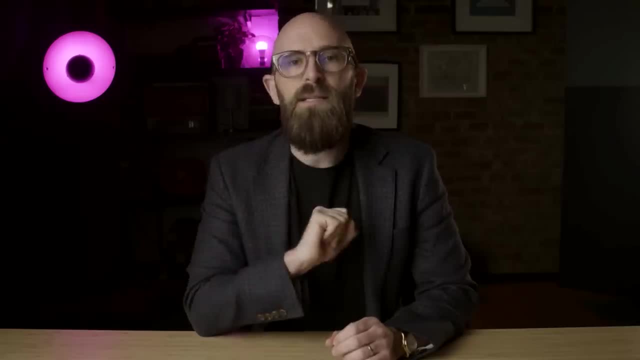 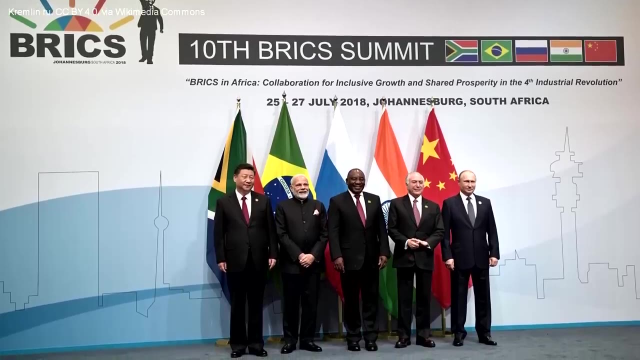 africa's lifeline. on august, the 23rd of this year, south africa signed a massive infrastructure overhaul agreement with china as part of the country's brick summit, also attended by india, russia and brazil. as part of the country's brick summit, also attended by india, russia and brazil. 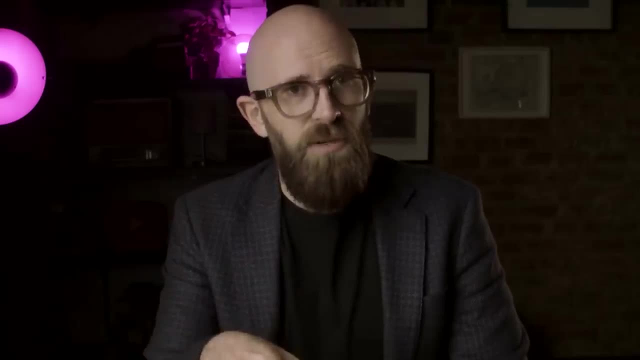 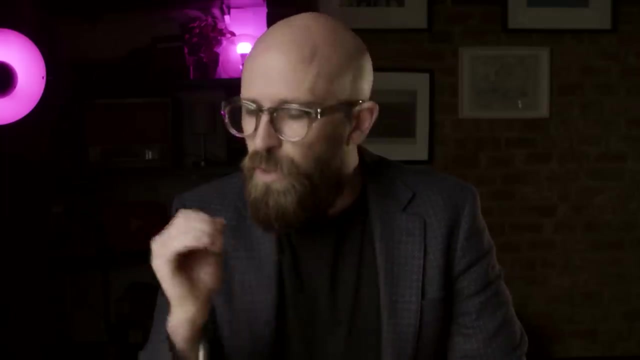 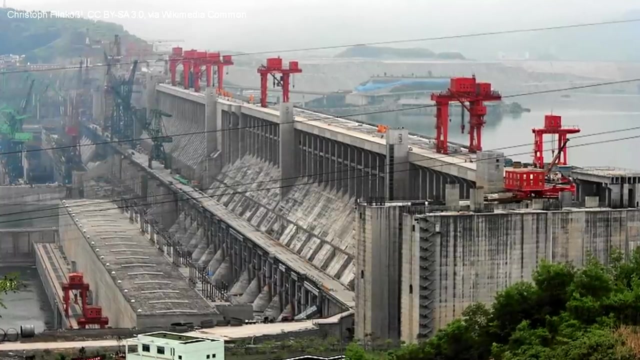 the deal would not only upgrade the nation's transmission and distribution systems, but bring much needed expertise in renewable energy plant construction and extend the life of the nation's existing coal-fired plants. add to that a series of grants and emergency power sources and china's resources, which south africa has now accepted. well, it's the sort of offer that a country in south 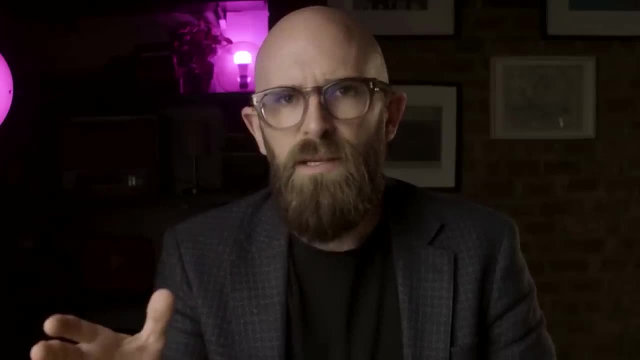 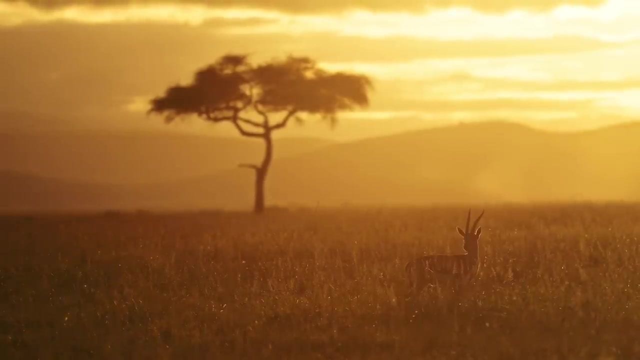 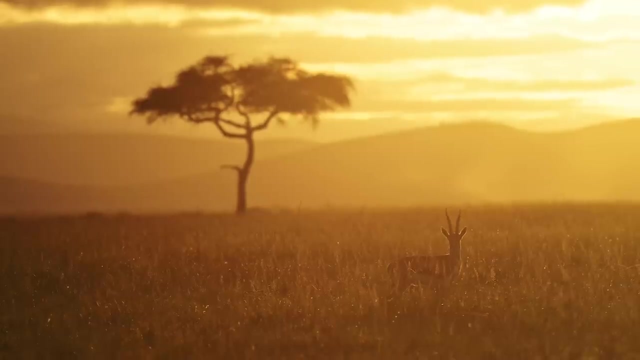 africa's position just can't refuse. the package of deals comes alongside a long-standing initiative of the indian national government to expand its influence throughout africa, leveraging diplomatic ties, deepening trade relations and sponsoring large-scale infrastructure projects as a form of soft power, bringing these countries under china's influence without having to take any 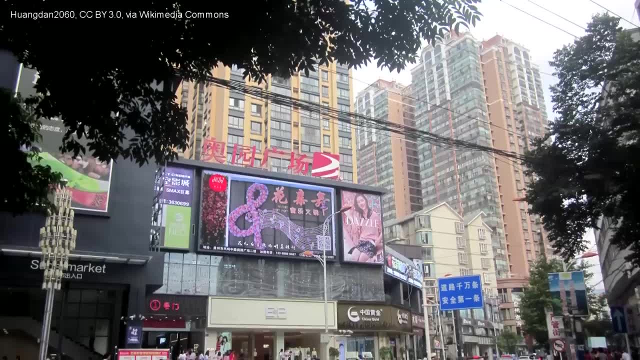 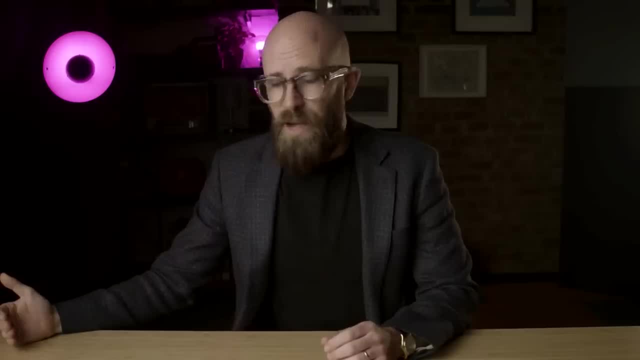 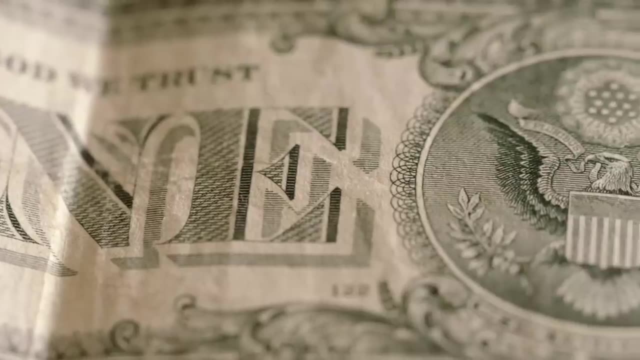 hostile action. china, and south africa in particular, maintain a booming trade relationship with china investing more into south africa than almost anywhere else in the world, even before this new aid package was signed. this sharply contrasts what south africa is encountered from the us and the in europe, who've been willing to supply funds in the name of moving south africa toward renewable 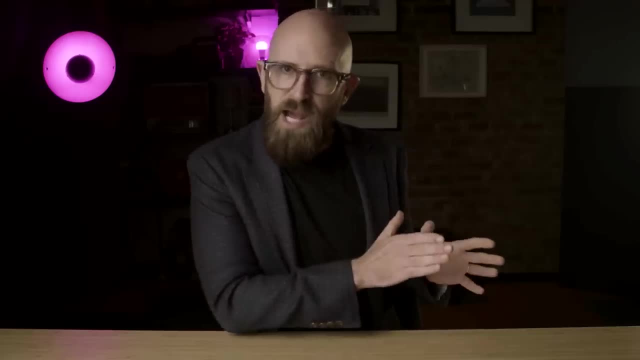 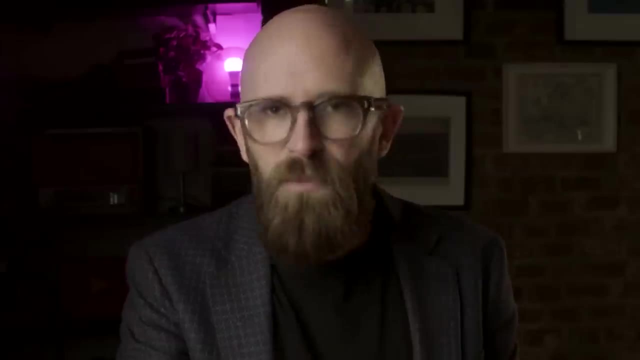 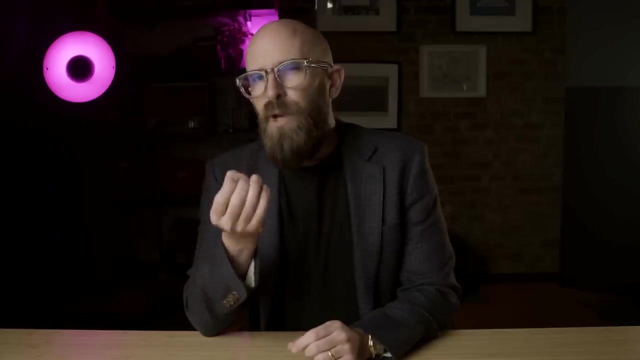 energy, but have been far more conditional in their support than china has, with south africa, strongly incentivized to take the most utilitarian solution as soon as it appears, simply to stop the bleeding. the global west simply cannot compete with china's willingness to provide help immediately. now, when trying to put our finger on what might come next for south africa, it seems at least from 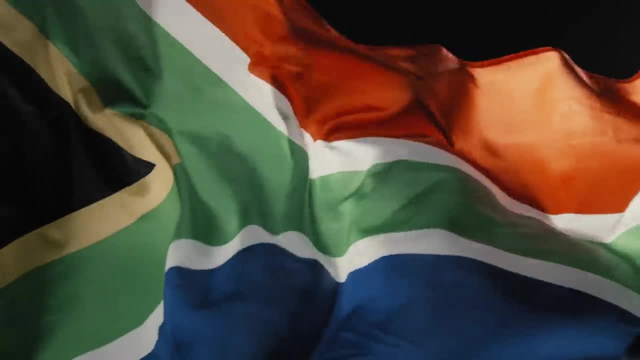 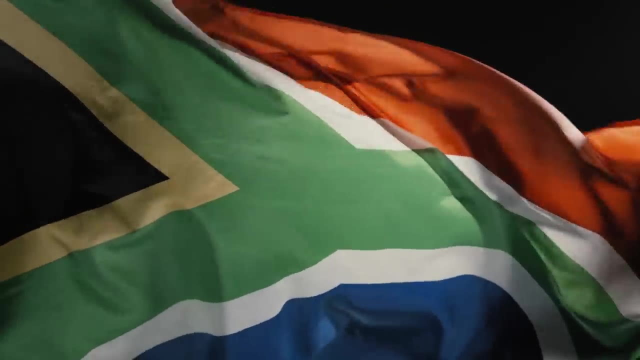 the outside as if things could go in a few different ways. there's the version where south africa gets itself together, either because of the actions of its federal government or in spite of them. there's the option where the nation relies on foreign partners to get through its lean years, and 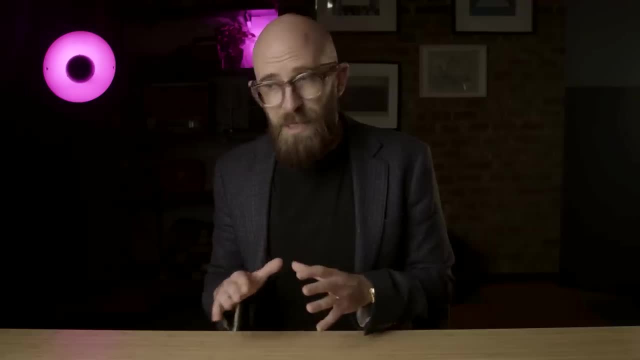 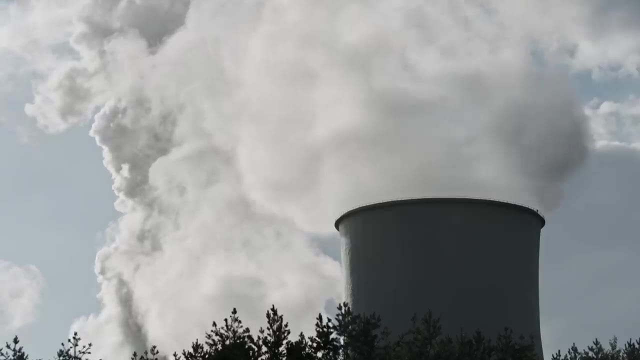 there's the worst case scenario, where this situation, already close to untenable, just continues to get worse in the coming years. south africa has pledged to phase out 12 gigawatts of coal power and replace it with 18 gigawatts produced by renewable sources. 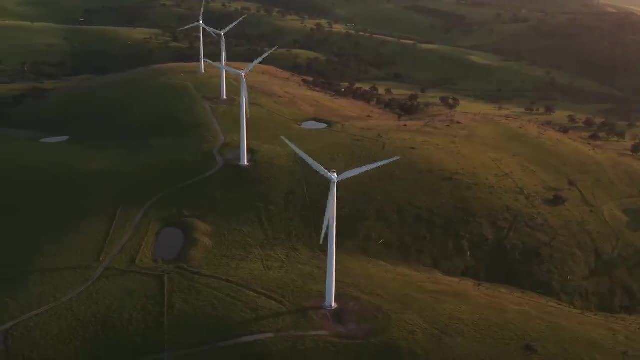 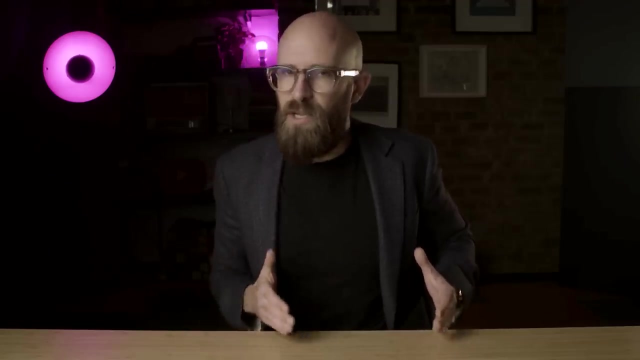 but even in this best case scenario, this is a process that takes more time than the people of south africa may have. it's an open question how many more grueling years of shortage the country can endure, especially given the effects of the shortage are getting worse each and every year. 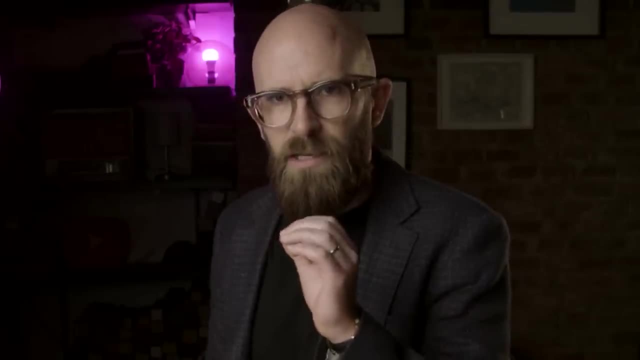 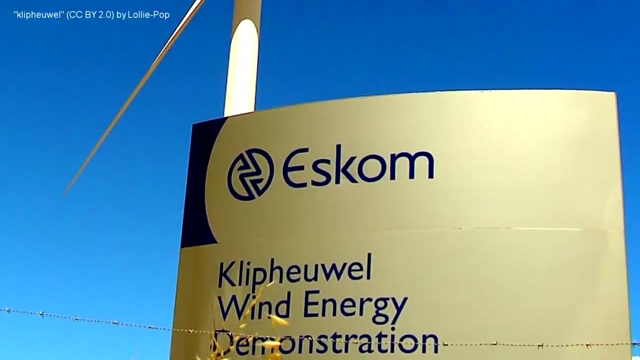 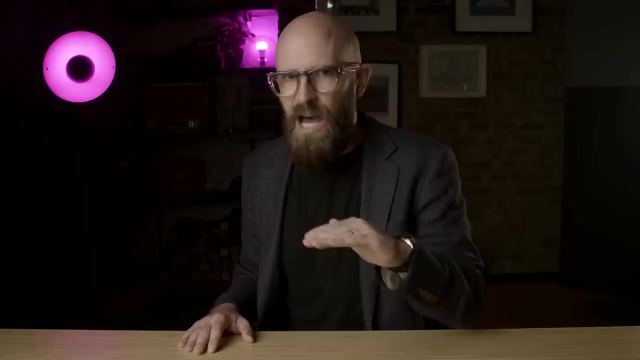 but there's also another dimension that we have to consider here, which is that at present, the creation of any new power plants of any kind are probably going to be done through escom, with the utilities track records. so far, especially with its more recent plan, there's no indication that south africans should expect anything other than an excruciatingly 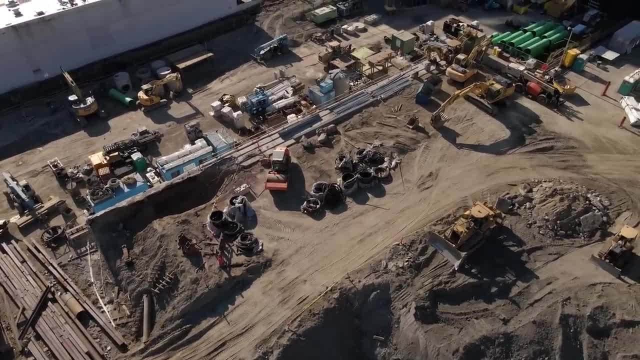 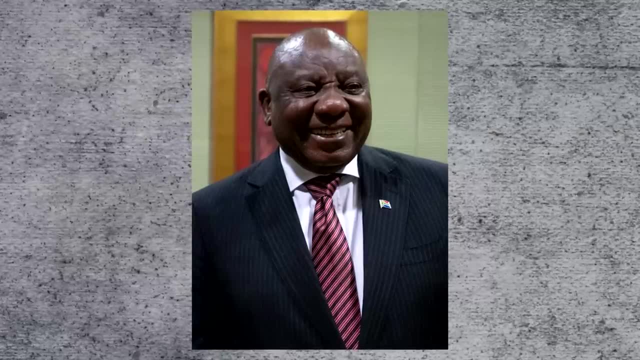 painful building process, and one that the country's elite will most likely use to enrich themselves yet again. south africa's current president, cyril ramaphosa, has emphasized his administration's desire to focus on the repair of the country's current coal plants and push off the dates at 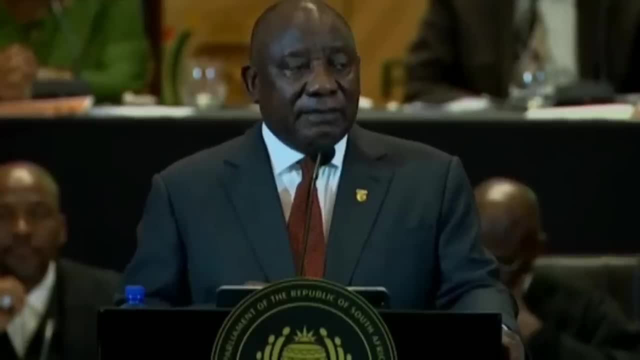 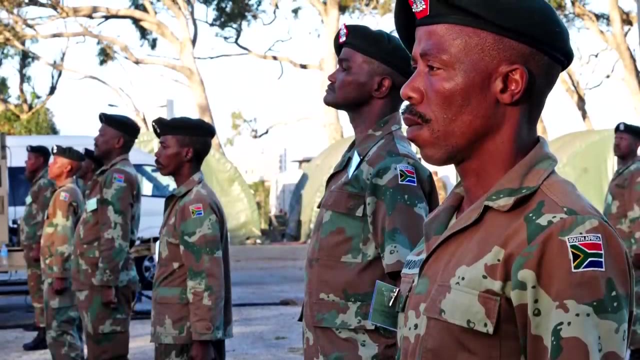 which others are expected to shudder completely. so too, as he declared a state of emergency to provide more unilateral authority in dealing with escom as a result of the shortage of coal power. indeed, he's mobilized the military to keep south africa's energy infrastructure safe, and he's 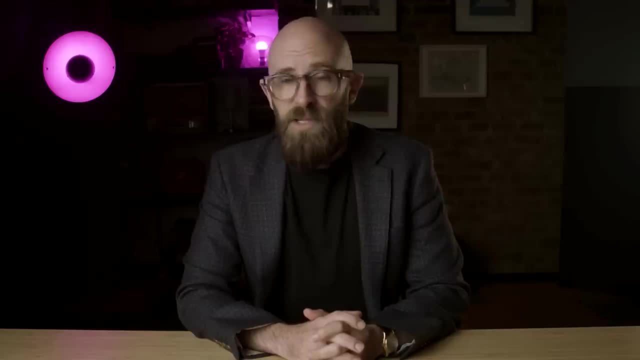 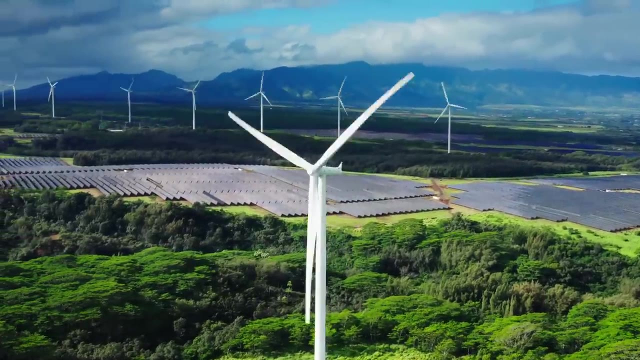 created a position in his cabinet for an electricity minister. the administration has also opened the floodgates to private energy development, stressing the importance of renewable energy in particular, and ramaphosa has thrown his personal support behind a breakup of escom. but in the grand scheme, a fair number of these initiatives have either failed to get off the ground or been ineffective once they did, while others are going to take years to implement. and still others are just a temporary stopgap. that may or may not be the case for the rest of the country in the near future. we'll see. 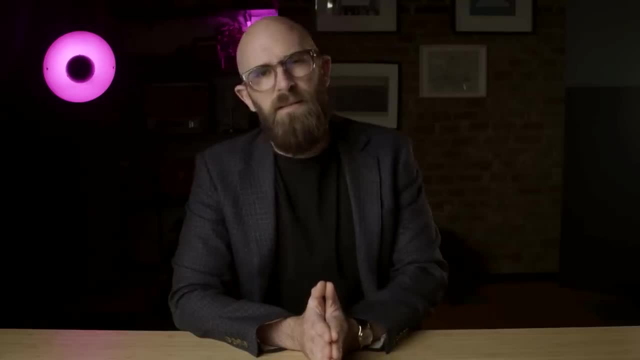 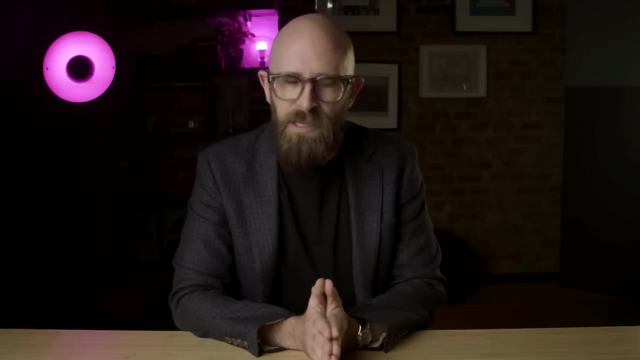 you in the next video may not last long enough to fill the void. in some ways, it's difficult to blame ramaphosa himself. his administration, after all, has inherited a long legacy of corruption and infrastructural inadequacy, but then again they inherited it from the prior administration, where ramaphosa himself 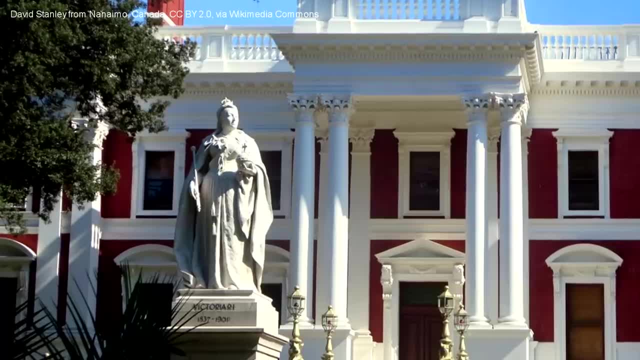 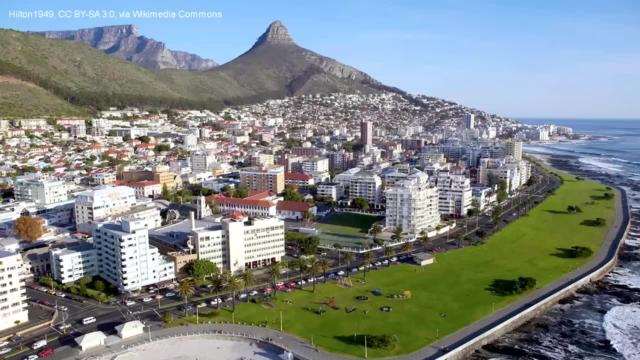 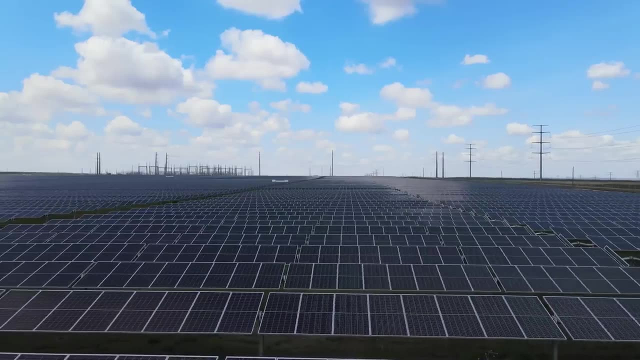 was deputy president, with few answers coming from the federal government. some cities and municipalities within south africa are beginning to explore other options. for example, the city of cape town has set a goal to go load shedding free within the next several years with the help of a planned solar plant that should provide up to 60 megawatts of renewable energy. not only 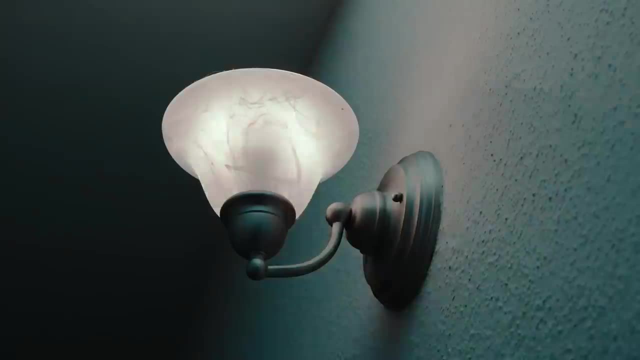 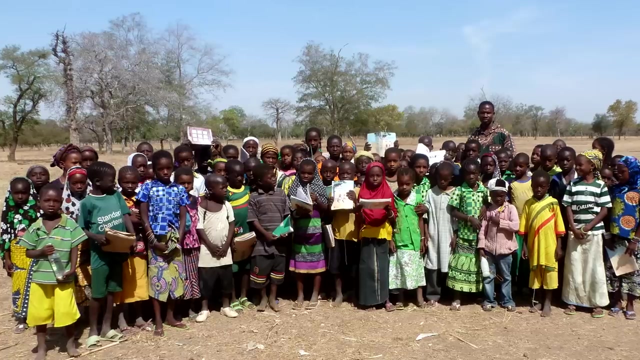 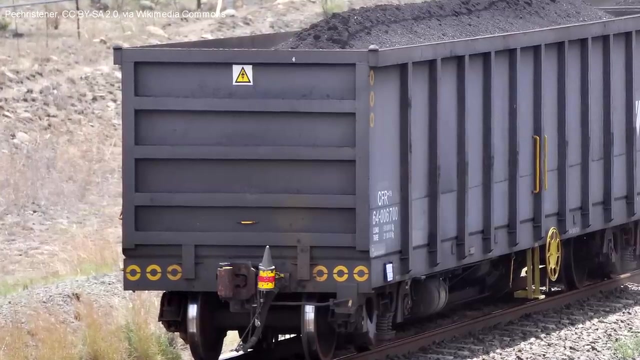 would this reduce cape town's susceptibility to blackouts? but it would have at least some effect in reducing reliance on the escom utility. the issue is whether such a change could ever be reproduced at scale, with south africa still economically reliant on the same coal industry that's slowly killing it. and then there's the implication of south africa's decision. 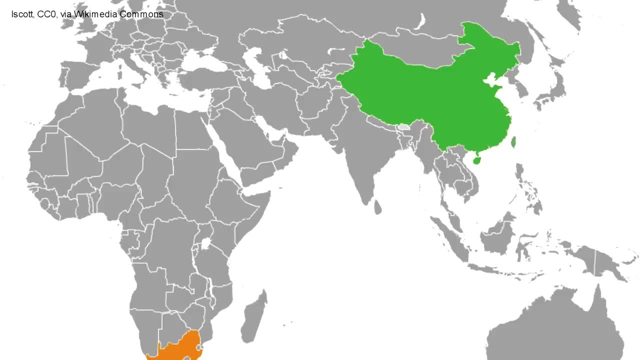 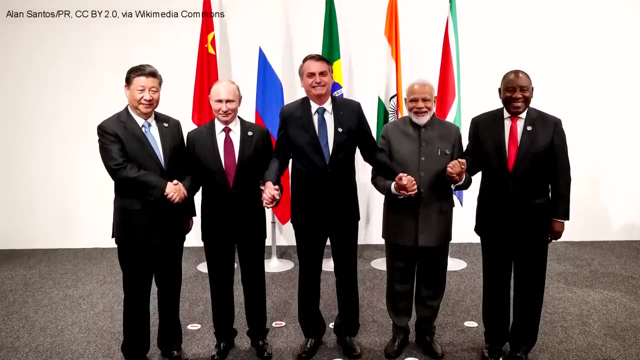 to strengthen its ties with china. as we mentioned, both south africa and china are going to have to work together to make sure that they don't end up in the same mess as they did in china. along with russia, india and brazil form a trade bloc called bricks, and it's possible that south africa's next 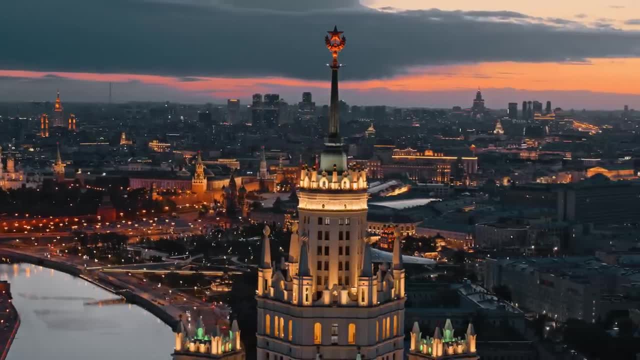 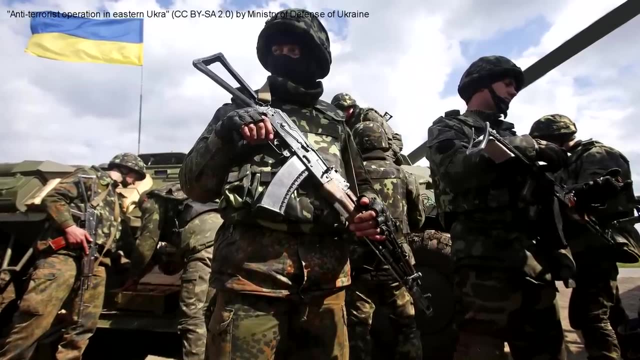 step might be to lean more heavily on the entire brick squad, rather than just china. south africa and russia already have a complicated relationship with south africa, unwilling to condemn russia's invasion of ukraine, and russian oil providers, particularly gazprom, all too eager to get their 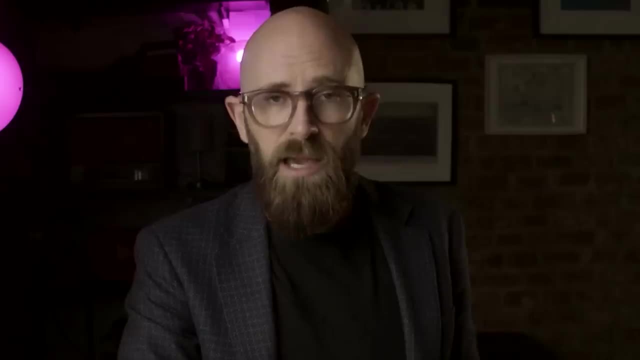 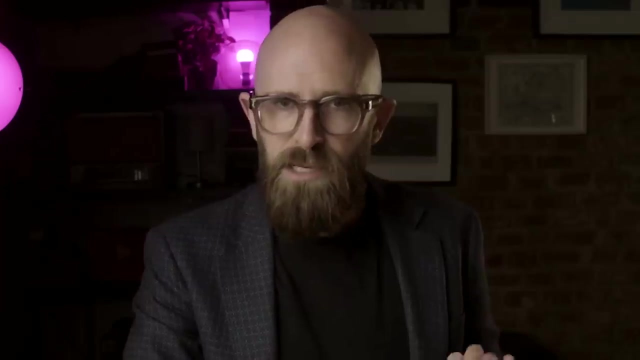 hands on a new customer to make up for lost revenues due to western sanctions. as we've seen between russia, china and a third nation tend to have some very real trade and political impacts on that third nation, something that south africa would likely need to weather as well. and lastly, 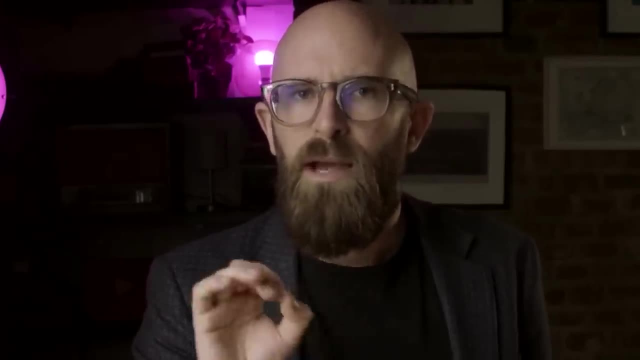 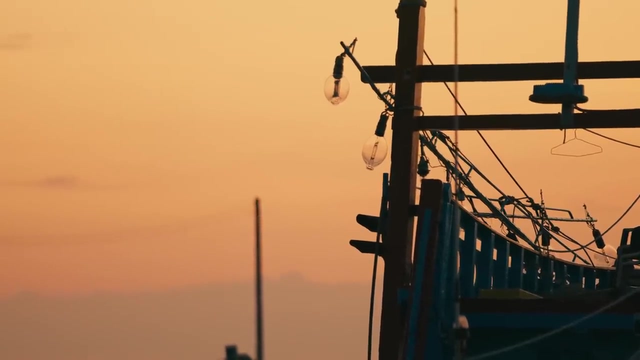 there's the outside possibility, the option that all of this plays out in its worst possible fashion. if the south african power grid cannot be rehabilitated in time, if the intervention from china doesn't come quickly enough or isn't comprehensive enough, it's possible that escom 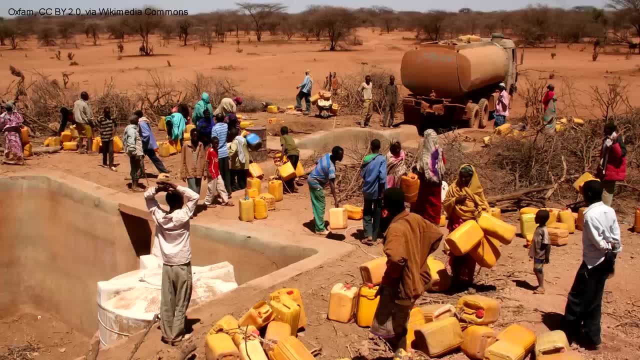 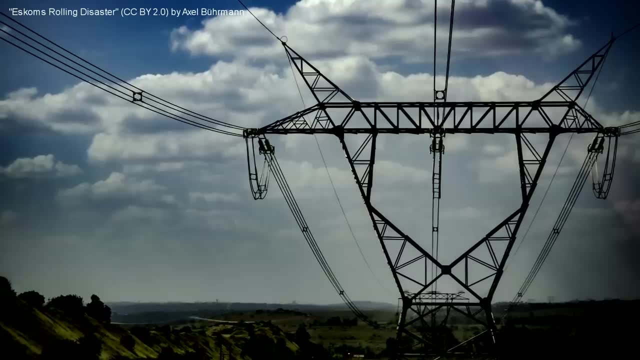 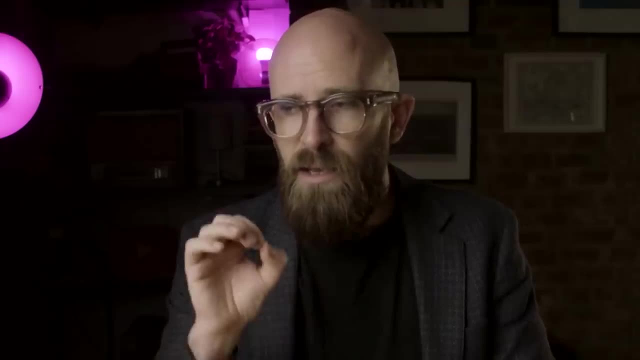 would be caught unprepared in the event of a major catastrophe- catastrophe from natural disaster to sabotage, to multiple co-occurring technological failures- there are a number of ways that south africa's grid could be pushed beyond the brink, and if that were to happen, then the ensuing collapse could get very ugly very, very quickly. take as a comparison: 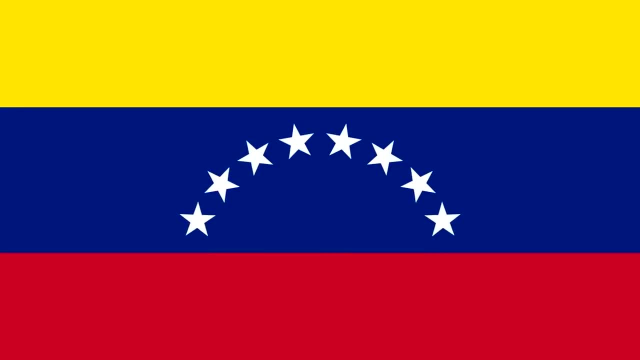 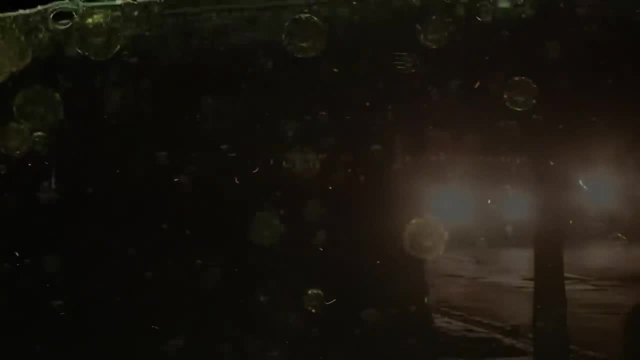 the country of venezuela, whose 2019 economic collapse was immediately precipitated by an energy crisis. unlike south africa, venezuela relied on oil rather than coal, but after oil prices fell to 8.2% in 2014, venezuela, like south africa, spent years trying to prop itself up rather than 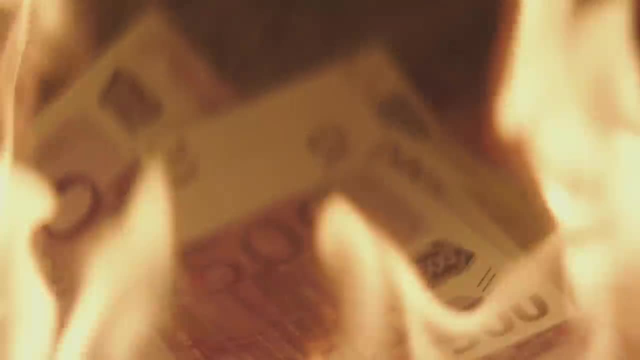 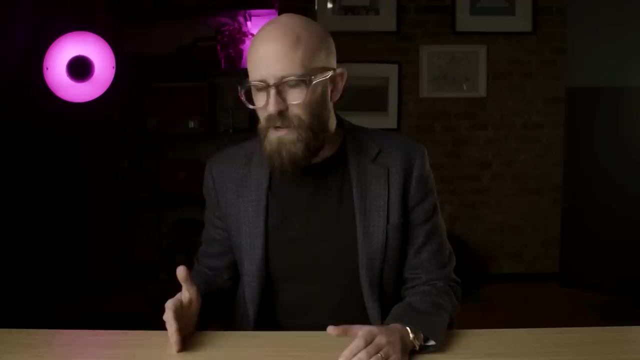 collapse completely. a free-falling economy directly led to lower oil output, sending the economy down harder, lowering oil output even more. when that crisis was combined with an unfair, undemocratic 2018 election cycle, the situation became too much to bear and since then, venezuela. 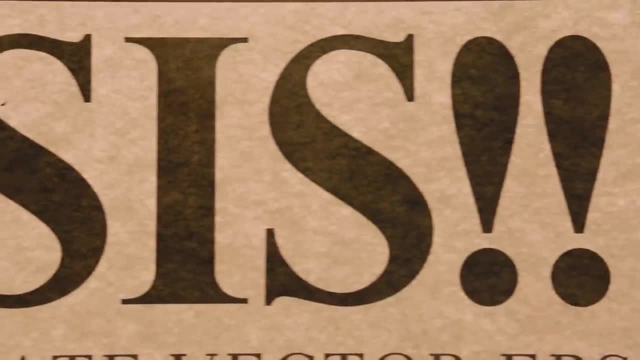 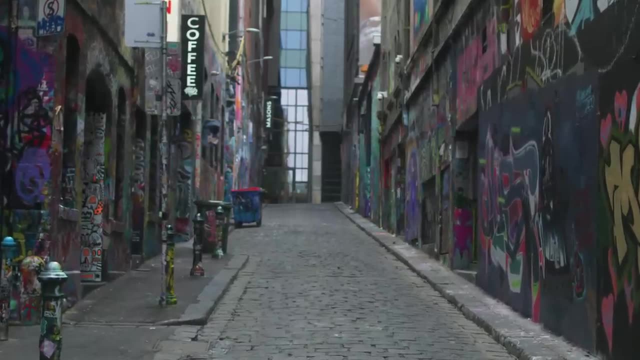 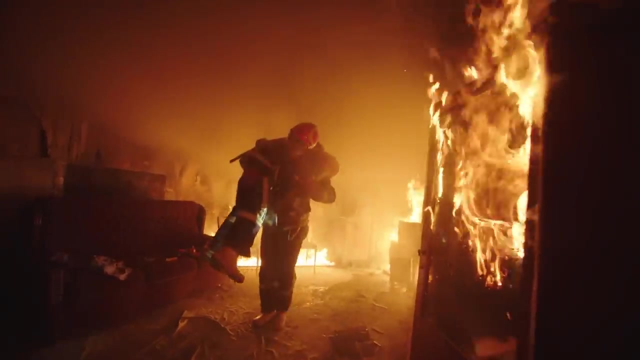 has been in complete collapse. in south africa, a country with, as we said, pre-existing high crime rates and endemic corruption, collapse could have dire consequences. first, the nation would likely face weeks of continuous power outage, during which time looting and public unrest would almost certainly rise to unprecedented. 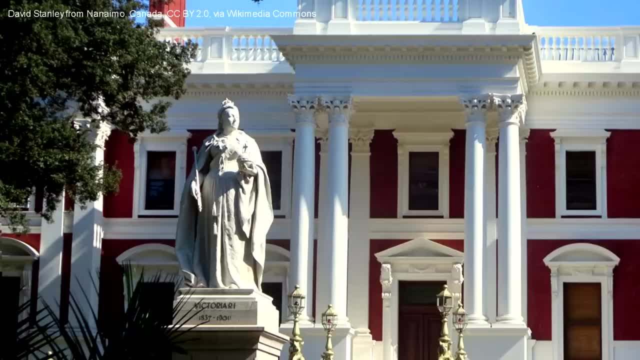 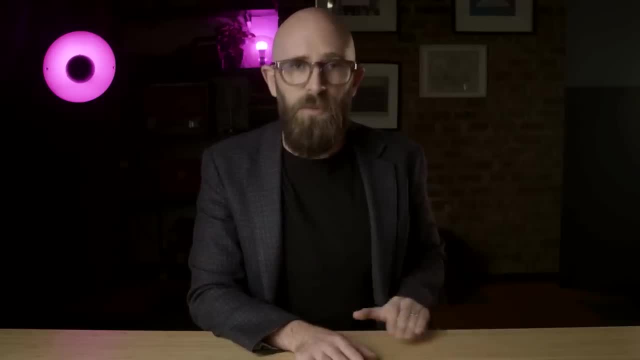 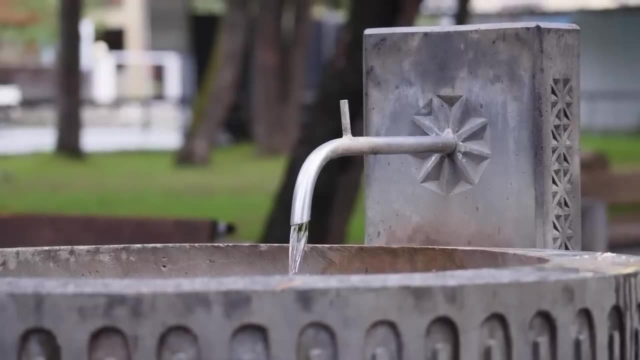 levels. at that same time, the south african government may choose repressive means to keep order rather than collaborative ones, especially in the event of either the african national congress or an opposition coalition getting a shaky or even illegitimate hold on power. the country's water supply and sanitation, already highly questionable, would likely go down the tubes. 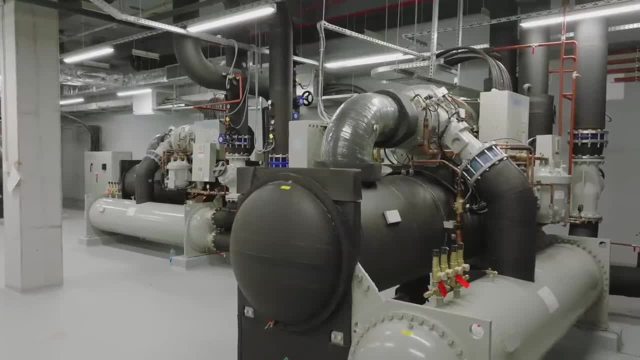 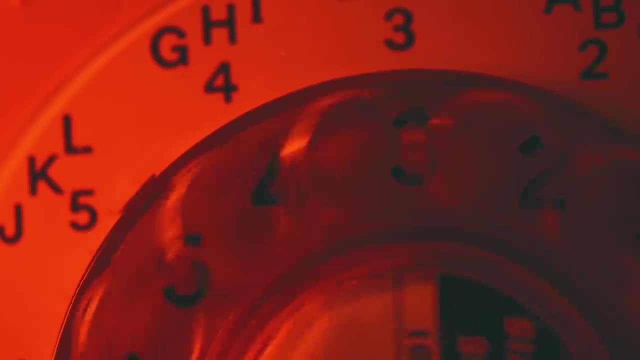 and as emergency generators run out of fuel, hospitals, morgues and food stores are likely to suffer catastrophic failure. south africa's telecommunication systems, just as reliant as anything on escon's power supply, would likely become inoperable and, according to escom's own 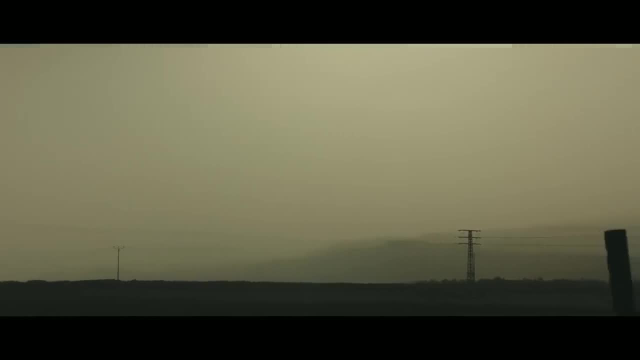 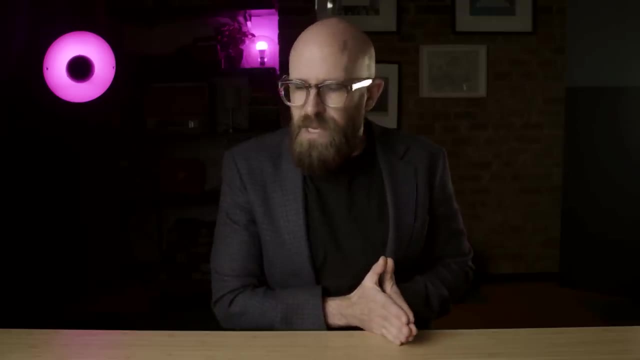 estimates their power grid could take as long as two weeks to restore. what that means and how it would be dealt with we can't say. but we've really got to stress that those in the middle of the media defects aren't just hypothetical. a present south africa's energy situation is such that the only reason why water and food haven't become unavailable, why civil unrest hasn't taken over and why hospitals can keep the lights on are the limited infusions of electricity that escom can supply. take those away and south africa will descend into chaos. perhaps that chaos is temporary. 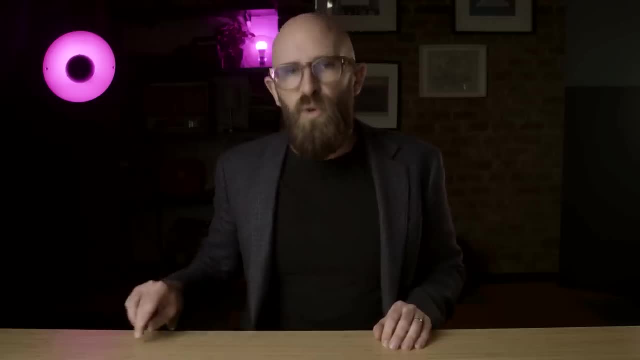 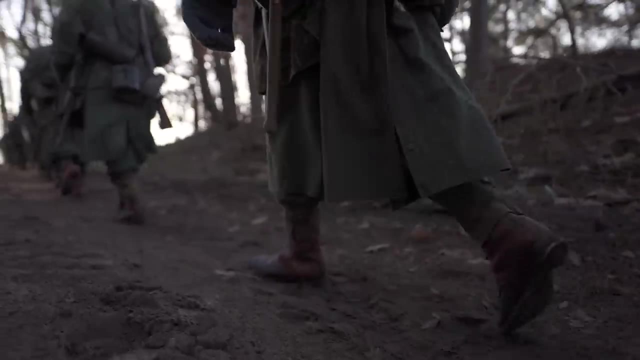 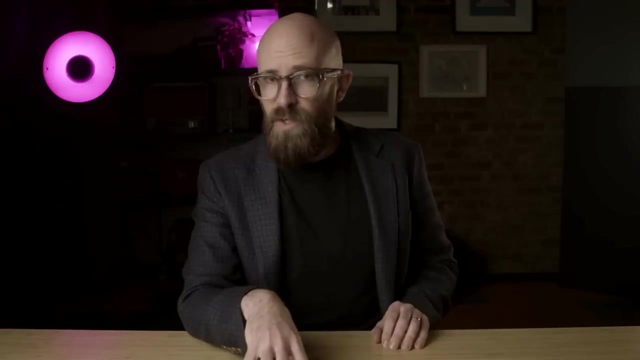 and power, then centralized authority is restored in short order. perhaps it would necessitate boots on the ground from china, from the surrounding nations or even from the west to lock down the pandemonium. or perhaps it leads to civil war in a relatively well-off nation that nonetheless remains deeply divided across society.